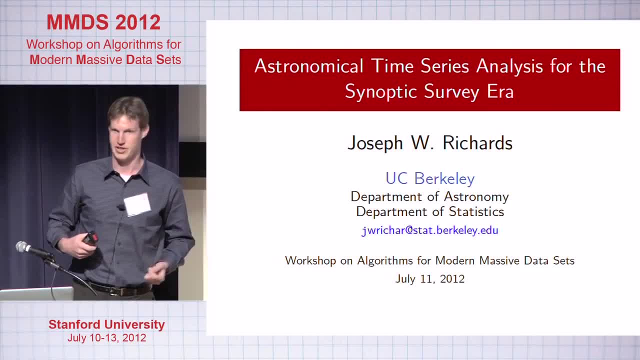 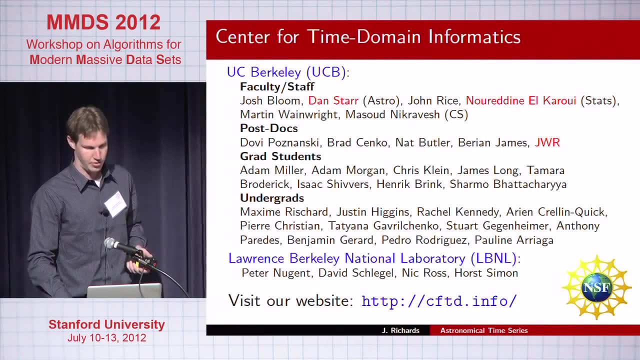 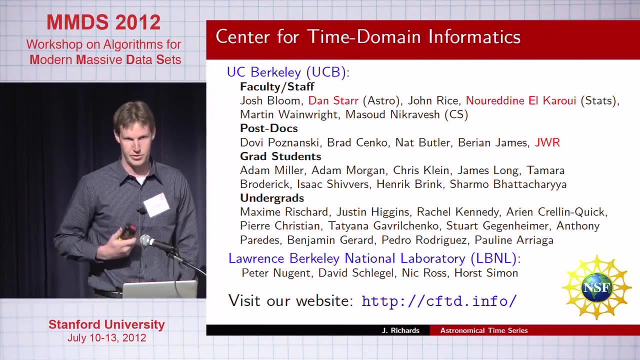 a static field, but monitoring the changes and brightnesses of sources- daily changes, weekly changes, monthly, yearly, et cetera. And so I'm a member of the Center for Time Domain Informatics. We are a collaboration of statisticians, astronomers and computer. 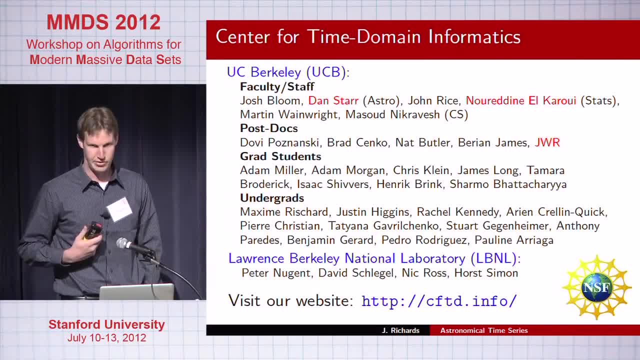 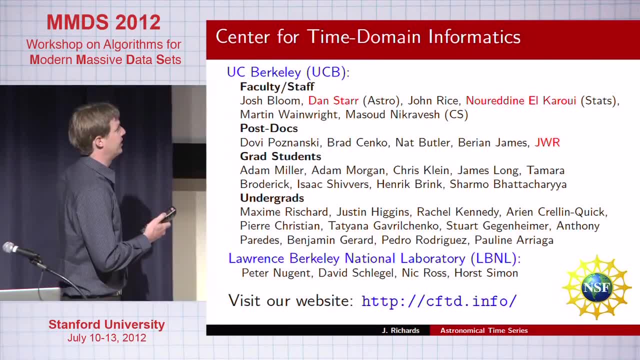 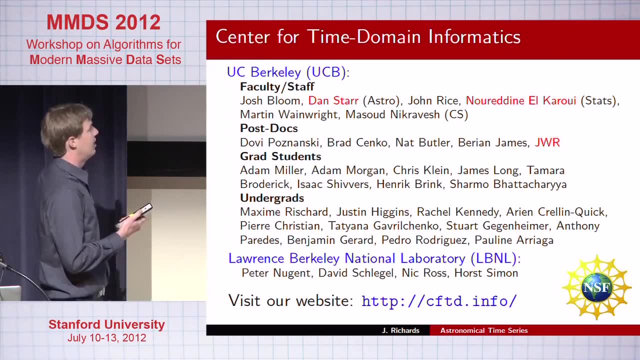 scientists at UC Berkeley and Lawrence Berkeley National Lab. The PI of the group is Josh Bloom. People in red are people attending the conference, So Nur ad-Din gave a talk earlier yesterday. Dan Starr, who does a lot of our database and engineering. 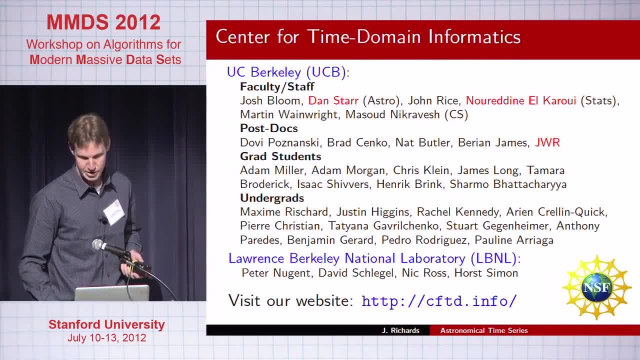 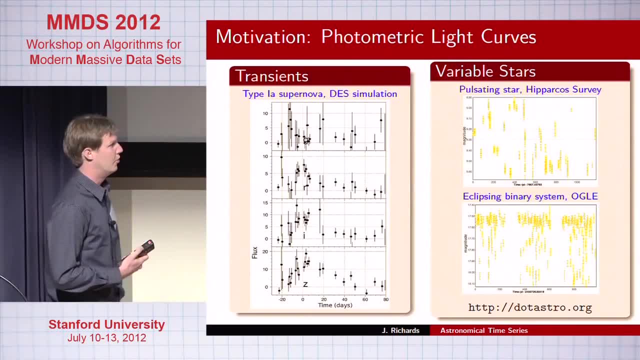 Dan Starr, who does a lot of our database and engineering work, has been in and out over the course of the week, So these are the type of data that we observe with modern telescopes in the time domain. What I've plotted here on the left is a simulated time series of measurements from a type 1a. 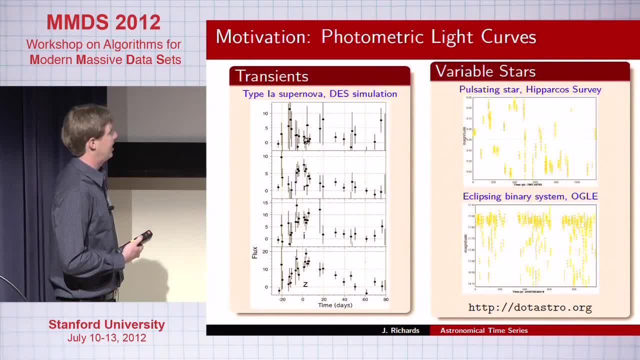 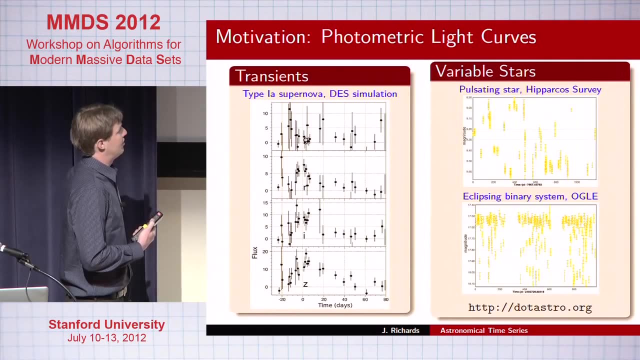 supernova, And what we have here is four simultaneous time series in four different optical photometric bands, And so you see that these observations are quite noisy. they're not evenly spaced. And you see, the supernova explosion comes with a rise of brightness and then a fall. 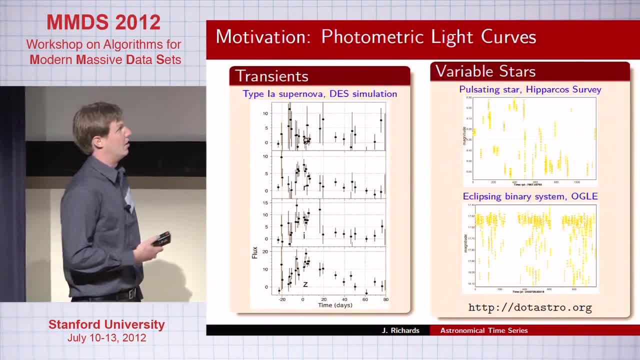 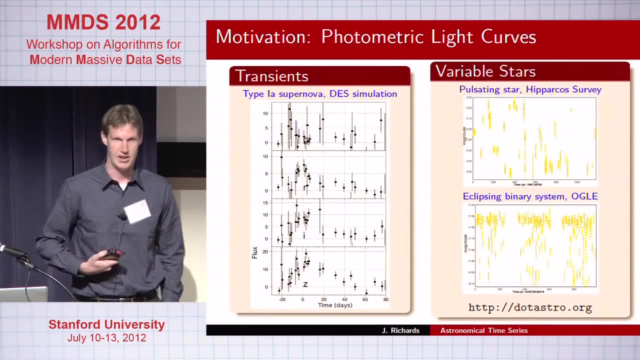 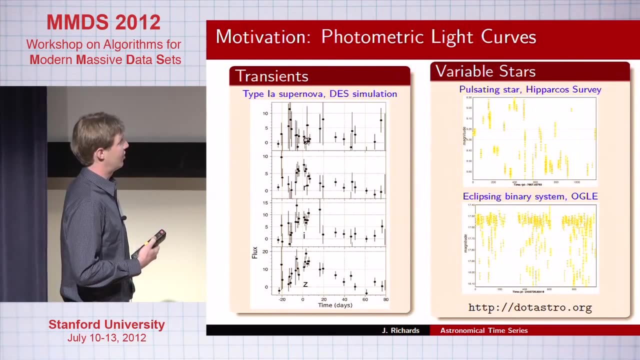 off and it doesn't return ever again. We also observe variable stars, which are objects that, for different physical mechanisms, change their brightness on timescales from less than a day up to a year. So this is a pulsating star. This is a CEOsUS. 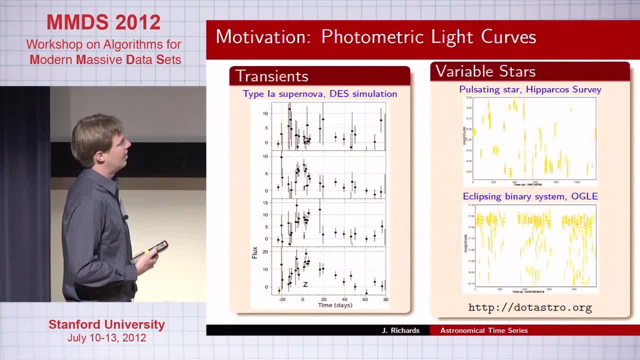 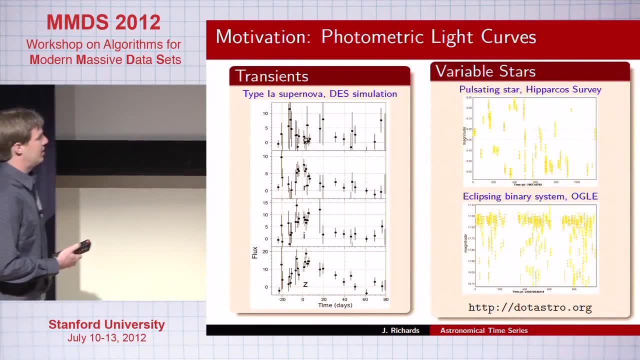 variable star, And again you see it's not evenly spaced data. If you were to phase this on the correct period of pulsation, you would see a nice clean curve, And so the idea is we're now collecting millions, soon to be hundreds of millions and billions of these. 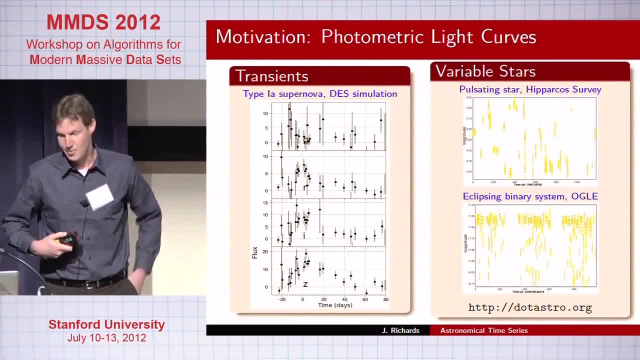 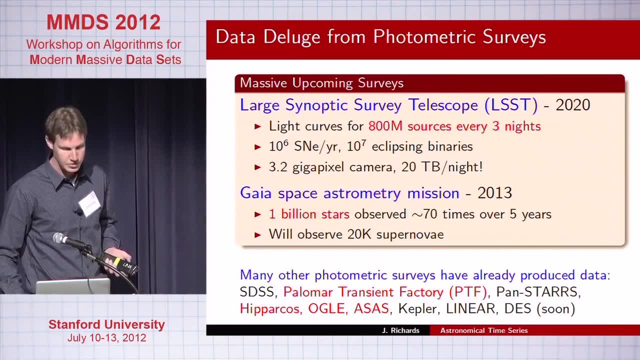 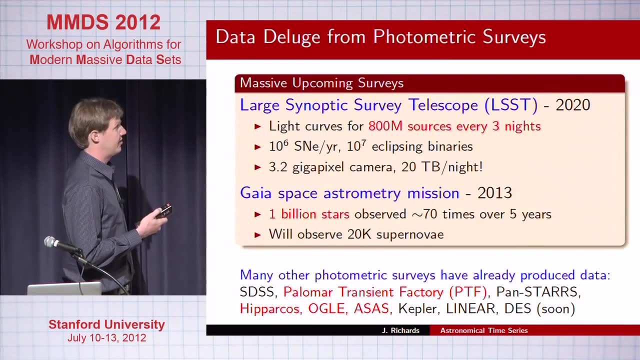 types of measurements on objects of up to hundreds of different classes of variability. At the end of the decade, as Alex mentioned, the large synoptic survey telescope, LSST, will come online And LSST is going to add a data point to each of 800 million time series. 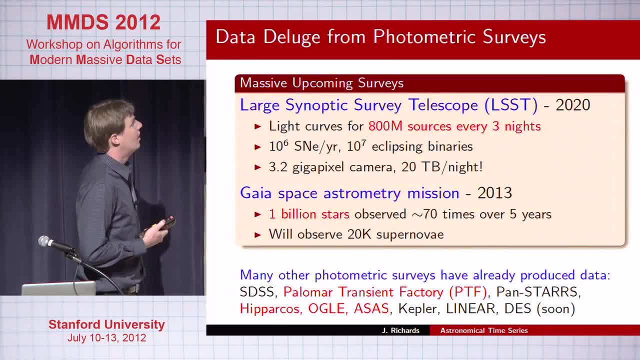 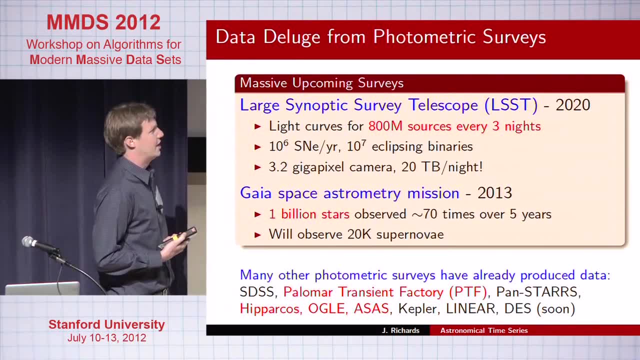 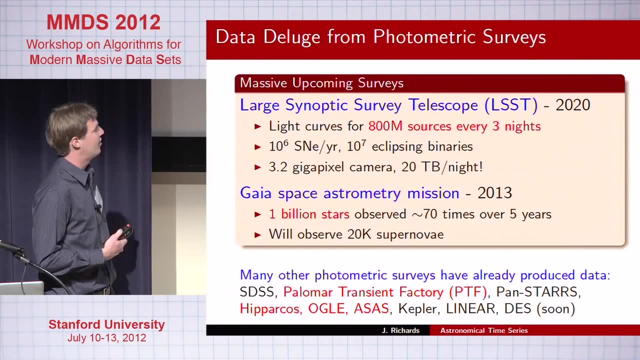 every three nights. That's a tremendous amount of data. LSST has a three-point point 2 gigapixel camera and we'll collect 20 terabytes of raw data per night, which is one slow and digital sky survey per night, even before we have the guys space. 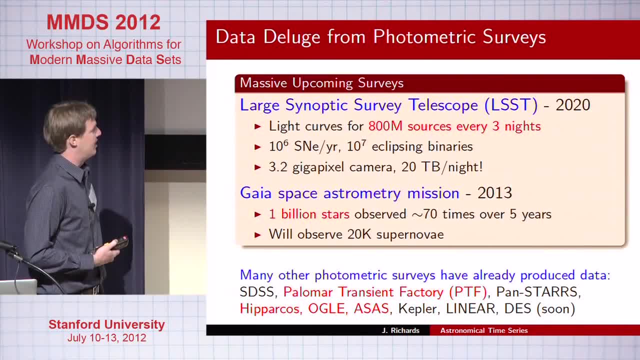 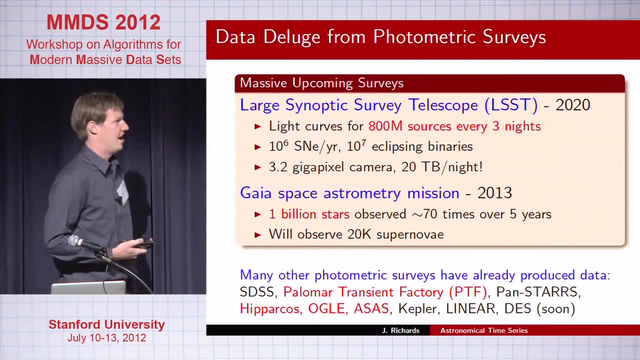 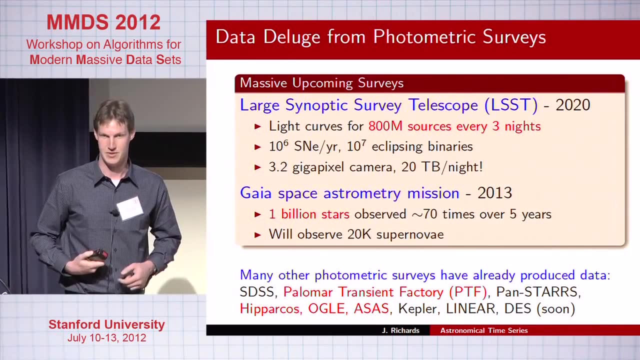 mission which comes online next year, and it will observe a billion stars 70 times over five years. and so we have this massive amount of information and our goal is statisticians and computer scientists- is to make sense of this data so the astronomers can use it to optimize their astrophysical and. 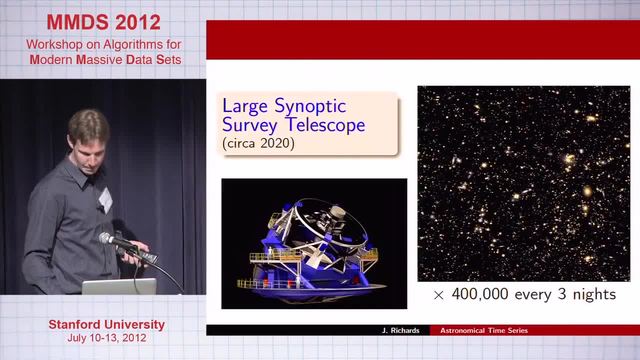 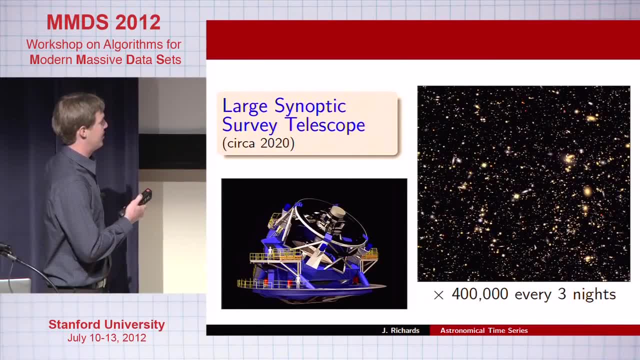 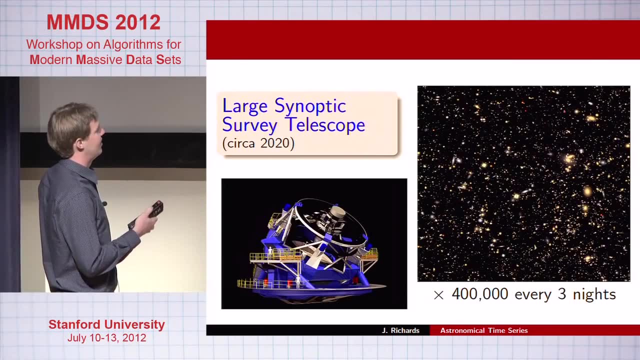 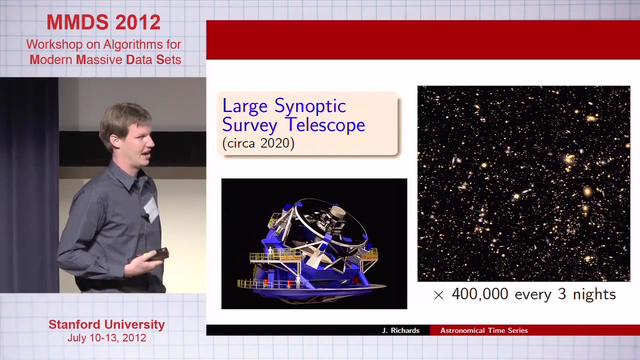 cosmological inferences. so here's a schematic of the else's تِ telescope for scale. this is a person right here. so LSST is going to observe something like this times 400,000 and then return to it every 3 nights. that will scan. 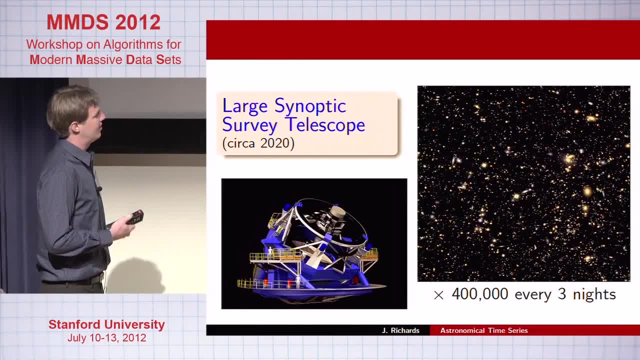 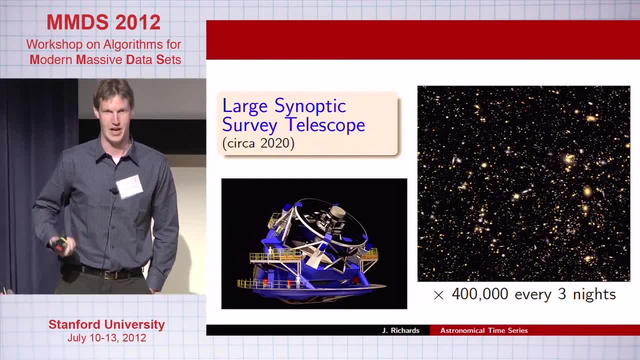 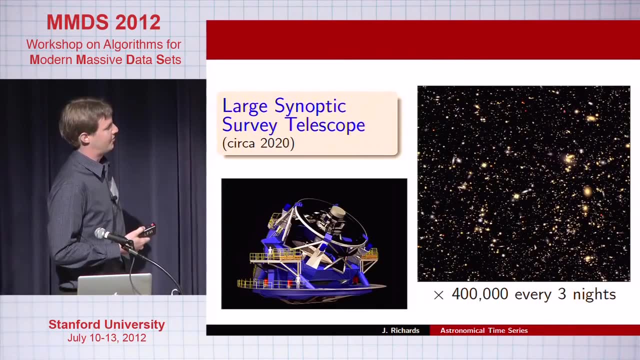 the show, entire sky, the entire observable sky. so what we see here is each of these little dots. the vast majority of them are galaxies, which may or may not host supernovae, which are exploding stars of different types. we also have a variety of different types of stars, and those stars may 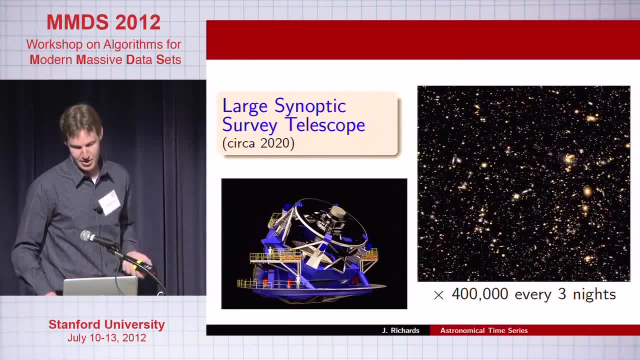 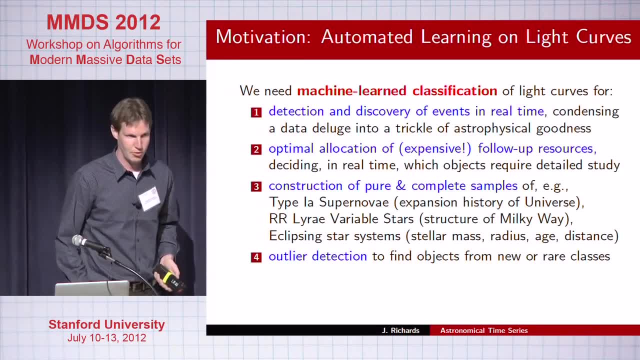 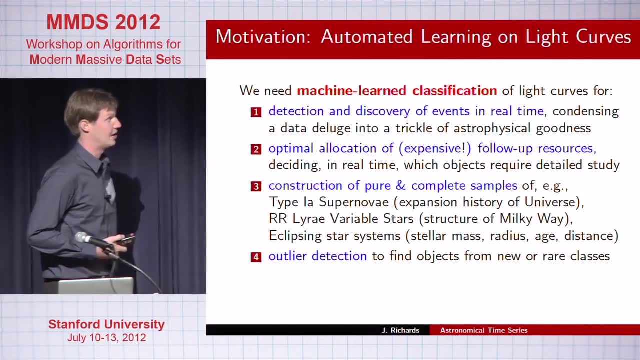 or may not be time varying, which may hold, which may be useful astrophysically. so, uh, in the business of classification of these time series, there's a variety of reasons that the astronomers are interested in this type of work. first is a detection of events in real time. 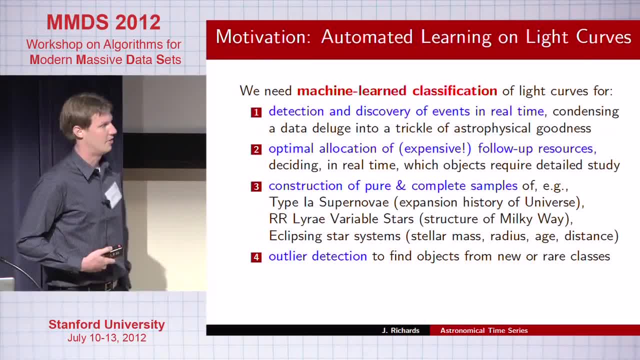 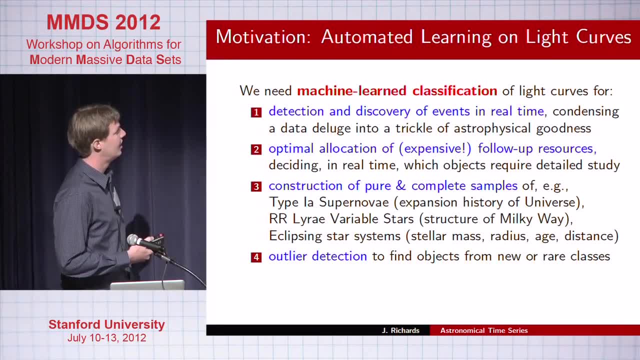 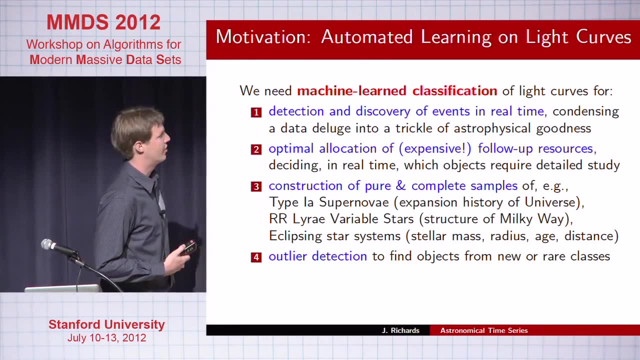 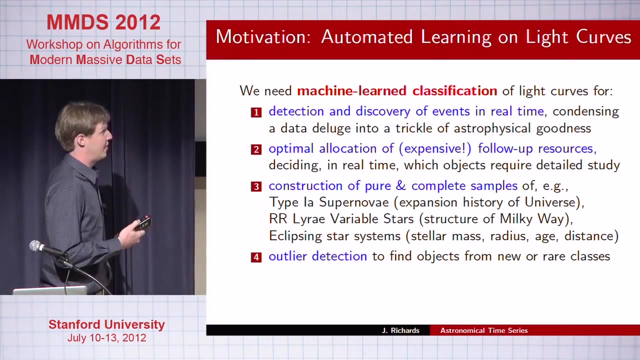 so by events i mean exploding things, things that occur and then maybe you can see their effects for a couple of weeks or up to a month and then never return, and this relates to allocating expensive follow-up resources to get precise amount of information on these objects. so alex alea was talking about galaxy spectra. spectra are actually extremely expensive to get. 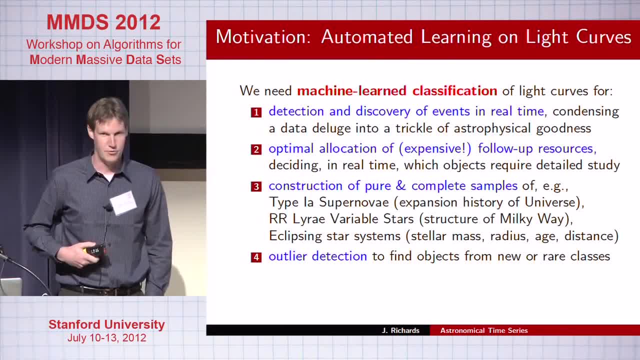 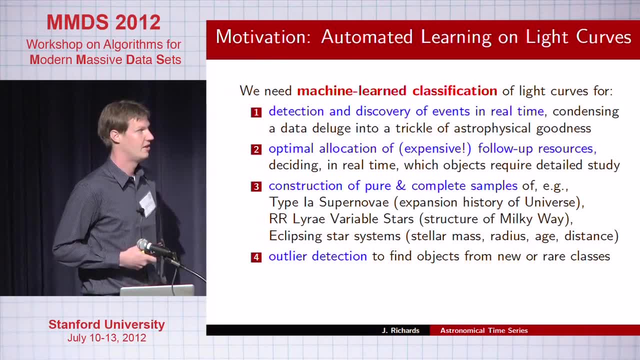 especially for fainter and fainter objects. so before we use one of the biggest telescopes in the world to observe an object, we have to be pretty darn sure that it's something of interest to us. third is to do classification, to construct pure and complete samples of objects. so for 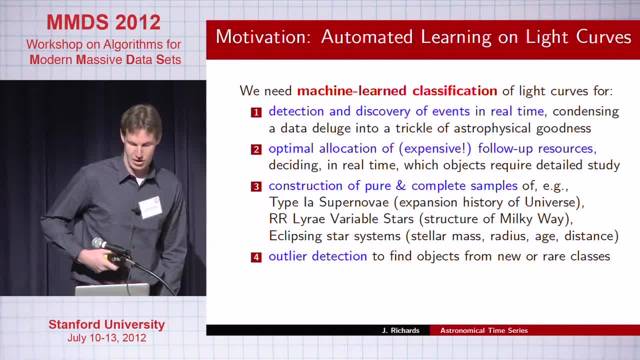 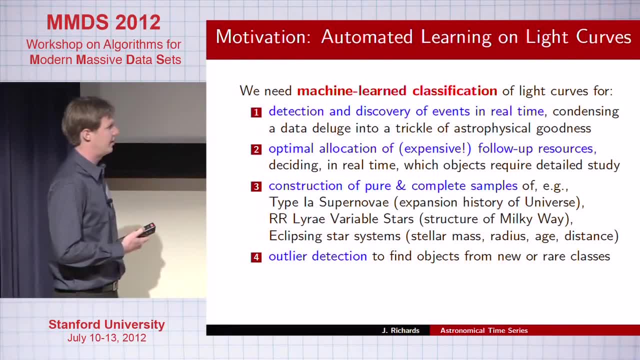 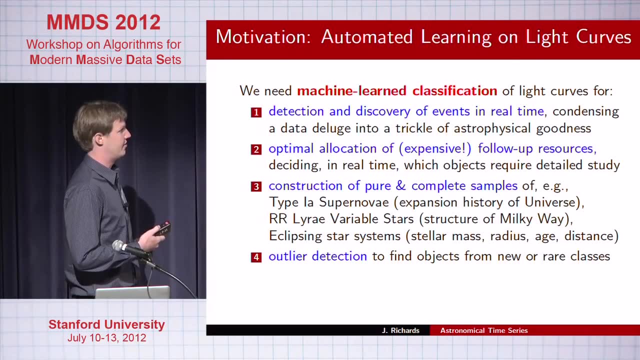 instance type 1a supernovae are are useful for doing cosmological research. the expansion history of the universe, so the accelerated expansion of the universe, was basically ascertained through a detailed study of the brightness of type 1a supernovae. there are other types of objects that are useful. 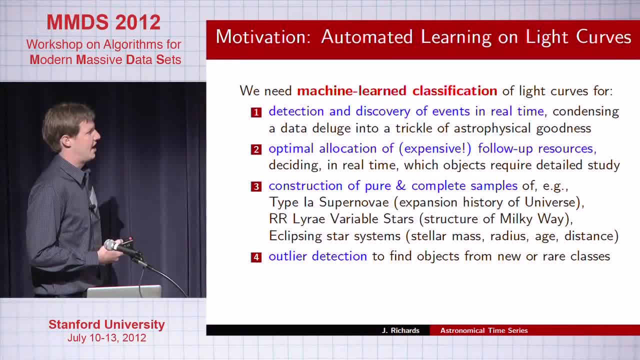 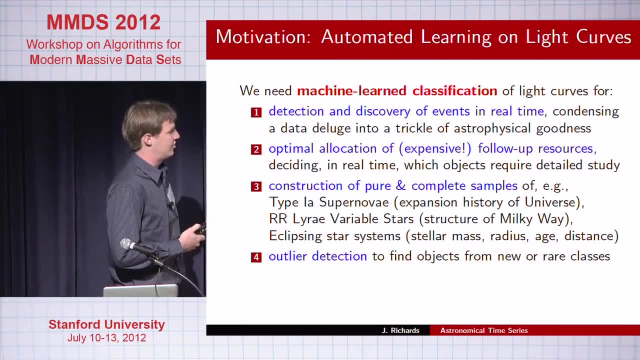 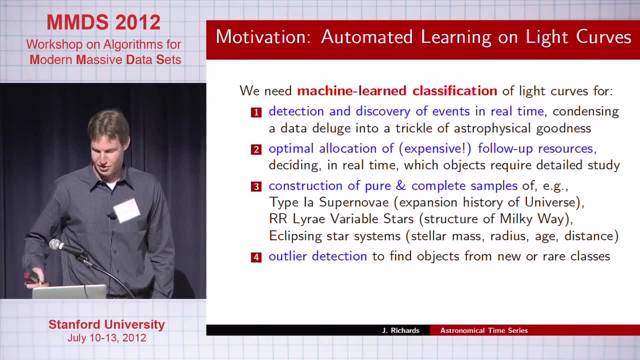 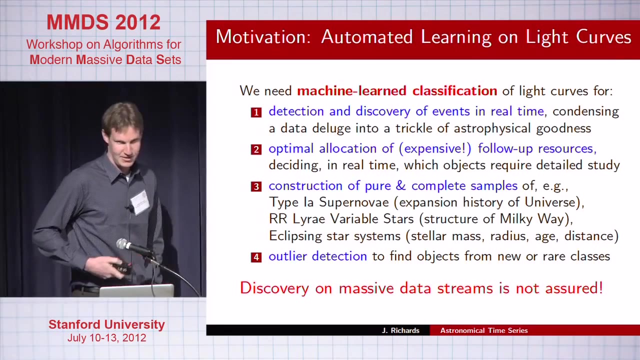 to probe the structure of our own galaxy, to understand basic physics in in the universe, and then, of course, outlier detection. some of the best and biggest physical insights are due to discovering new classes of variability and try to figure out what's going on in those. And so just because we have an LSST coming online, 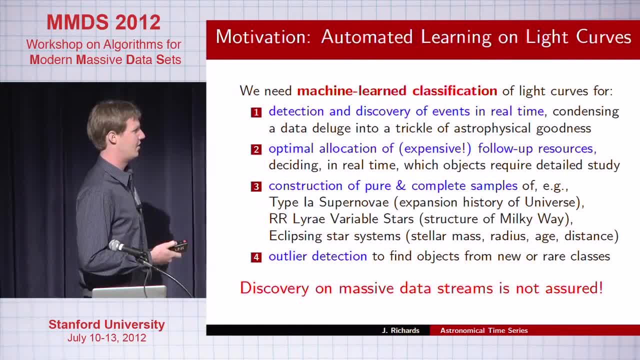 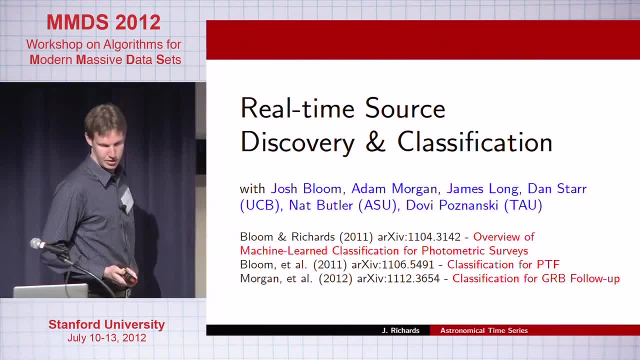 producing all of this data does not mean that discovery on these types of data streams are assured. So for the first part of this talk I'm gonna talk about kind of the real time classification work that we're doing, And then for the second half I'll talk about more. 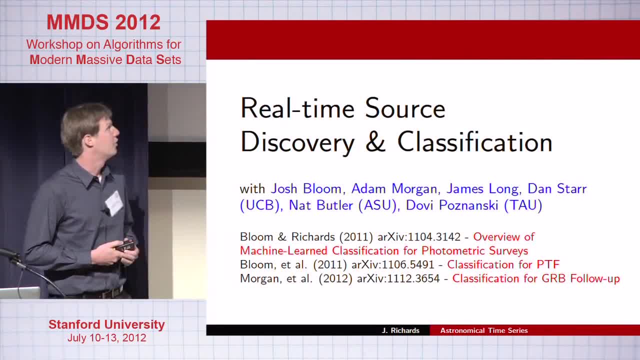 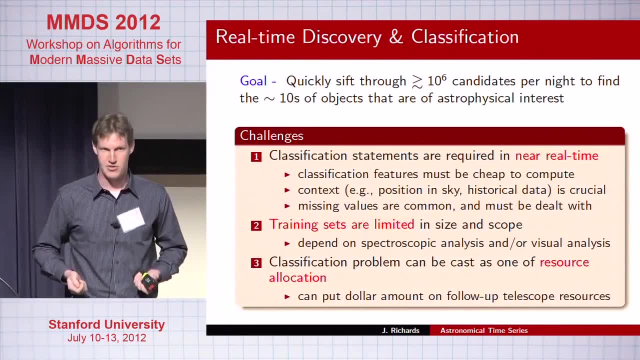 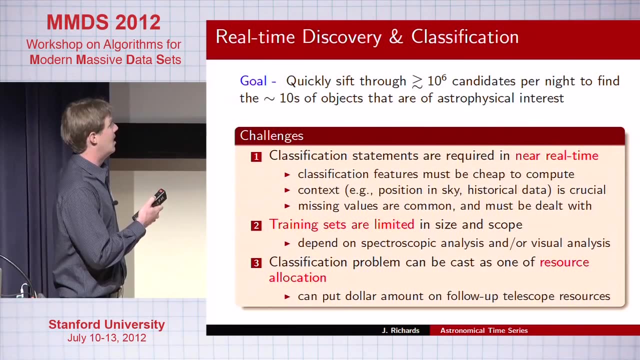 what I call retrospective classification, And so for real time discovery, we're really interested in allocating follow-up resources as quickly as possible on the objects that we care about. The goal is to quickly sift through upwards of a million. So right now, with a telescope that we work with, 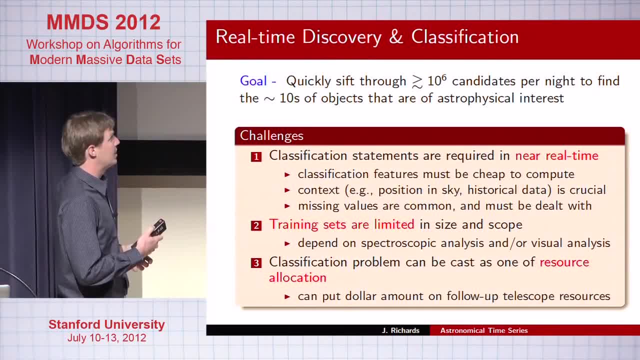 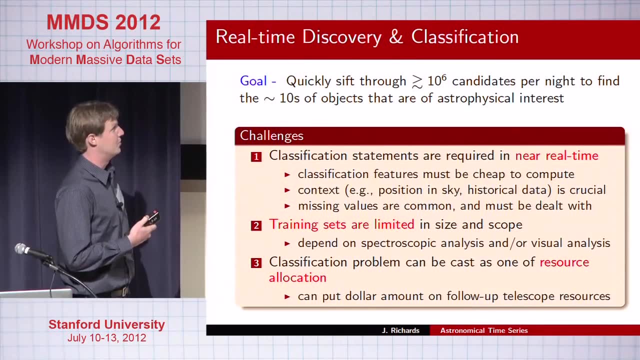 called the Palomar Transient Factory. we have about a million supernova candidates per night And for each one we wanna know which are the kind of tens of objects out of those million that are actually interesting to us. In the future that number's gonna climb to. 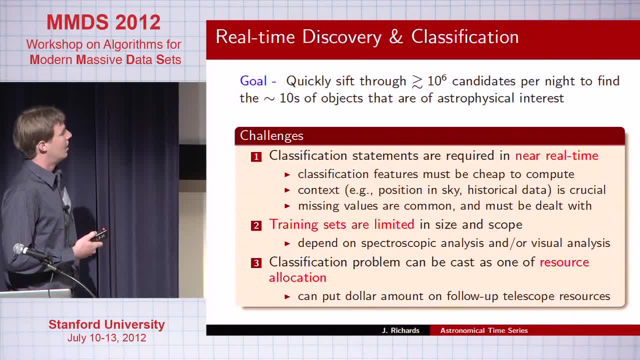 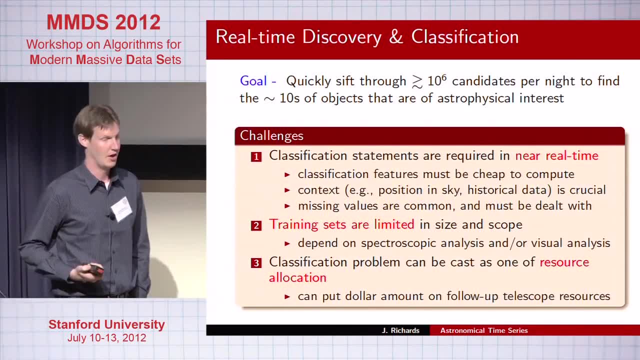 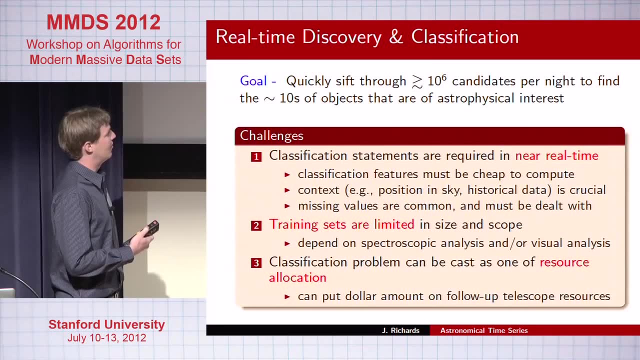 several orders of magnitude larger, And so we need near real time classification. So it's not maybe the real time that some people in this room are used to. We're talking about minutes to hours turn around time. So we need classification features on the two dimensional. 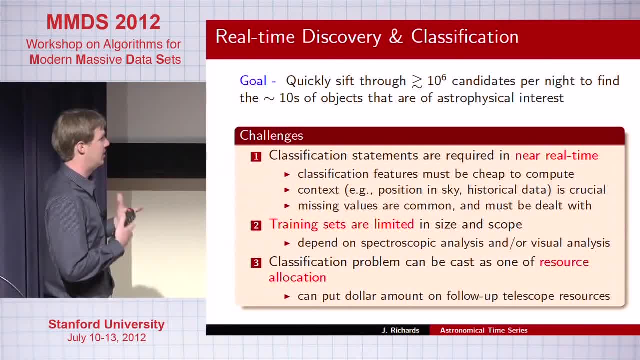 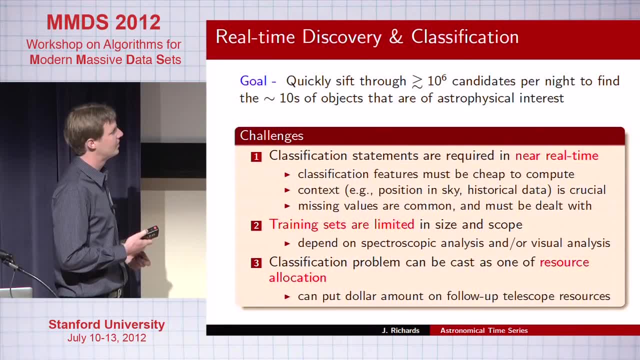 images which are used to produce a time series, And then the time series themselves Context information. so where is it? Is it close to a galaxy? If it is, it's probably a supernova. Is there historical data out there? Missing values are extremely common. 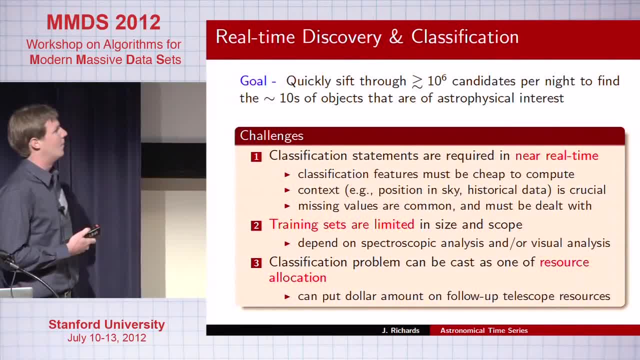 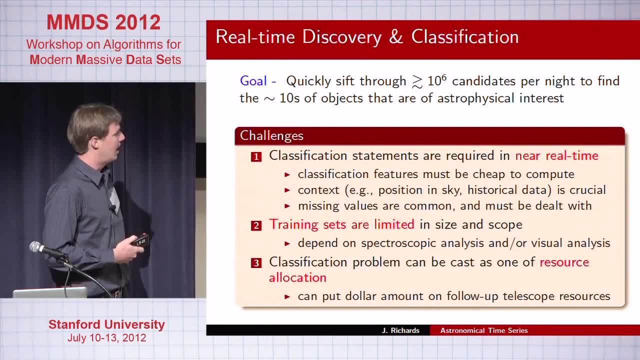 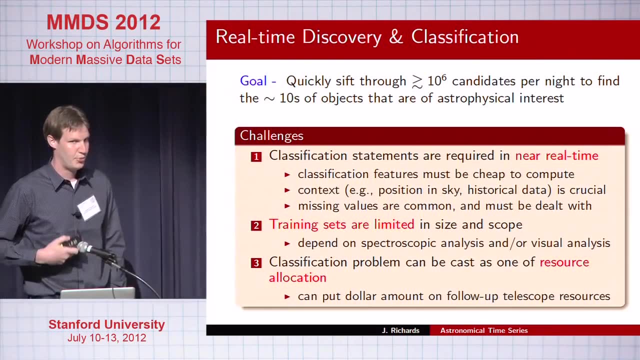 Bad data is extremely common and must be dealt with. We're really limited by both the size and scope Of our training sets. And then, as I said before, what really drives all of this is resource allocation, And since we can actually put dollar amounts on, 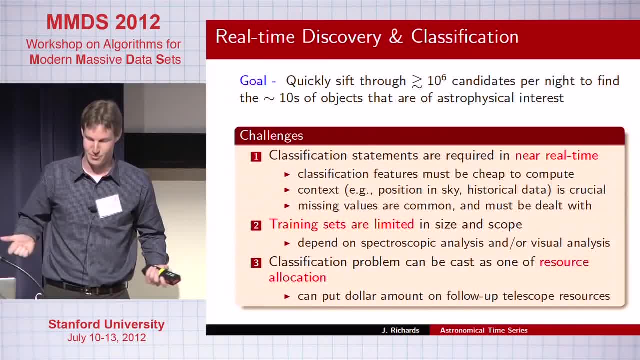 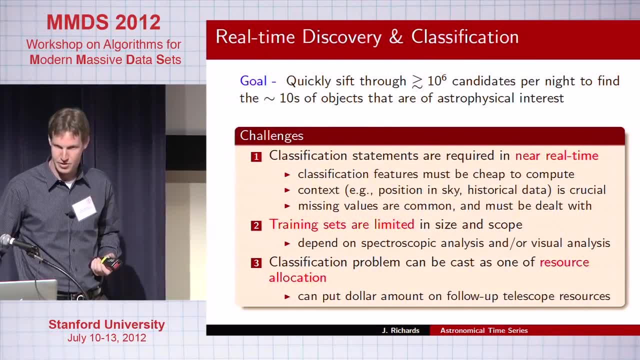 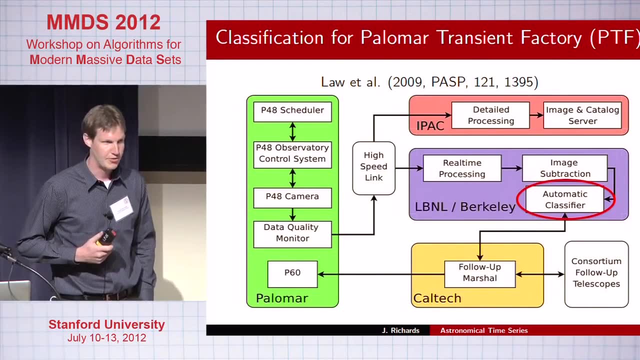 amount of follow up observation time on, say, one of the biggest optical telescopes in the world. we can actually phrase our classification performance in terms of telescope resources. So I'm also a member of the Palomar Trust, Palomar Transient Factory Collaboration. 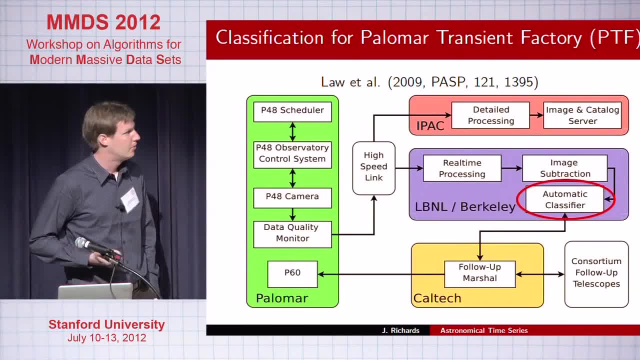 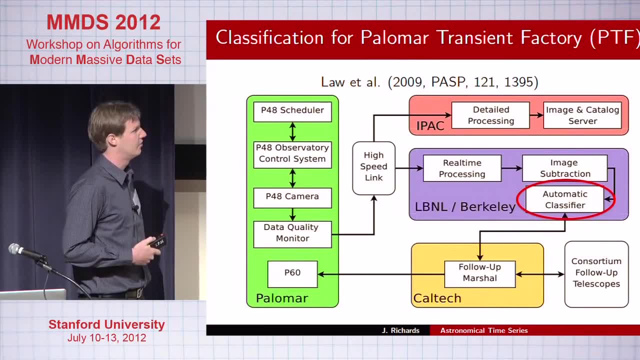 And so this is a project out of San Diego, in Palomar Mountain, And through two plus years of operation we have observed and spectroscopically confirmed almost 1500 different supernovae, Which is an order of magnitude more than what was known previously. 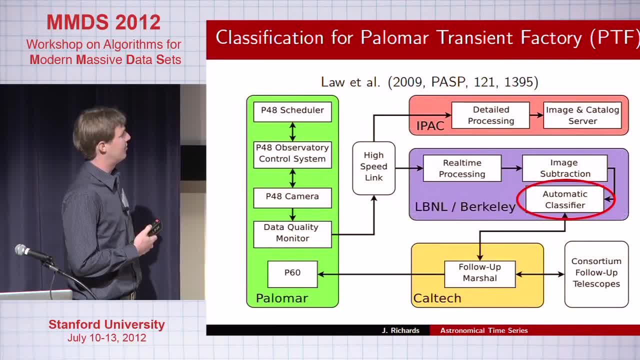 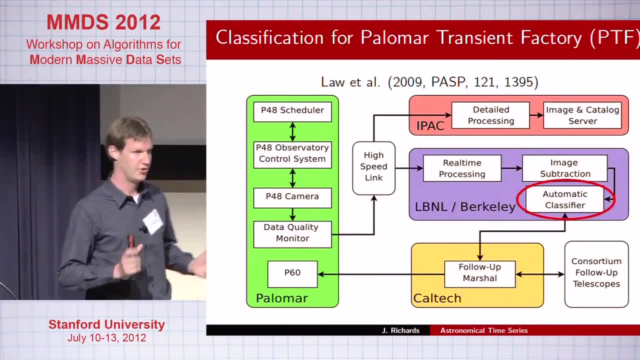 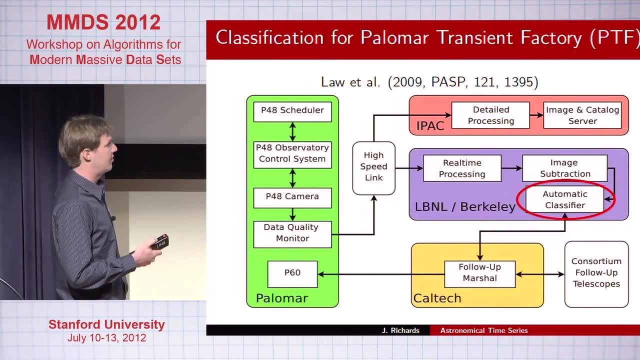 And so the basic data flow. at Palomar is, there's a 48 inch survey telescope which is continually monitoring the sky and producing images. Those images are then sent to LBNL, where they're subtracted against a deep reference image. 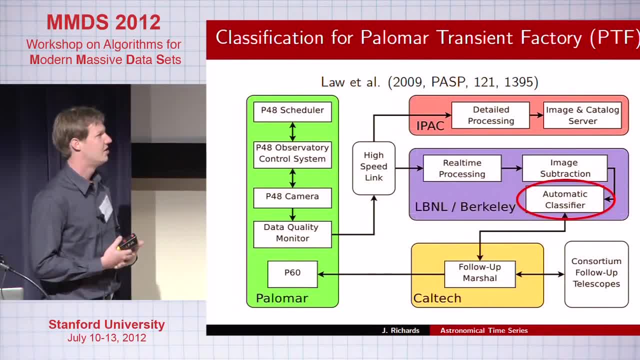 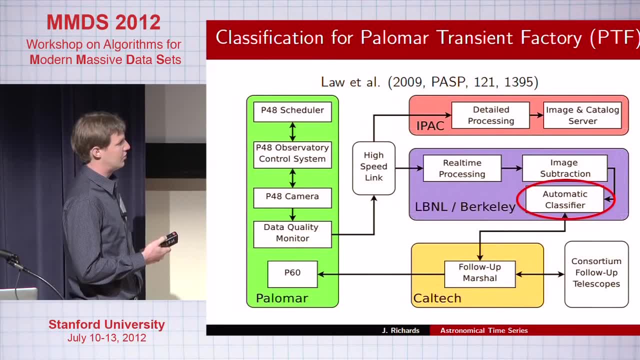 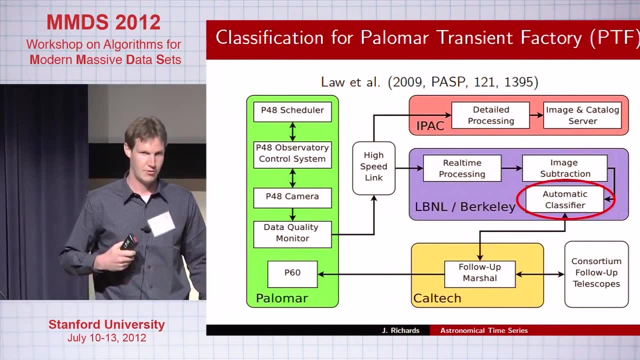 So basically kind of a median averaged image from historical data And those subtractions and the references are sent to us where we do classification, And the classification is kind of two-step. First is separating all the artifacts from the real things. 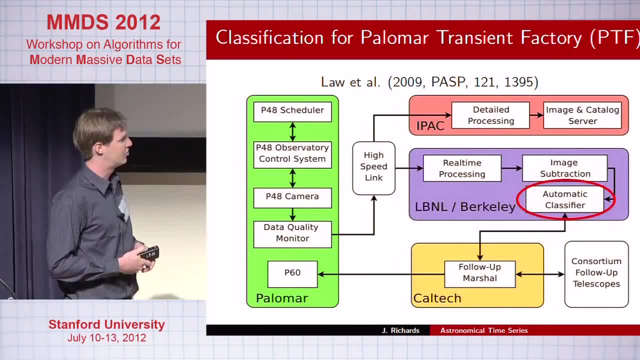 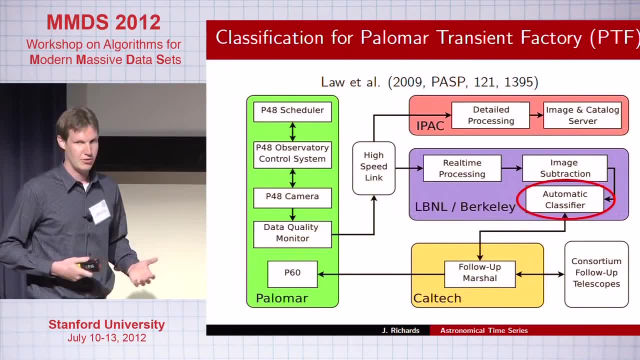 The truly astrophysically varying objects, Which is about a thousand to one ratio, artifacts to reals. And then secondly, once we know it's real, we want to know: is it a supernova, is it a variable star? So supernovae will explode and never come back. 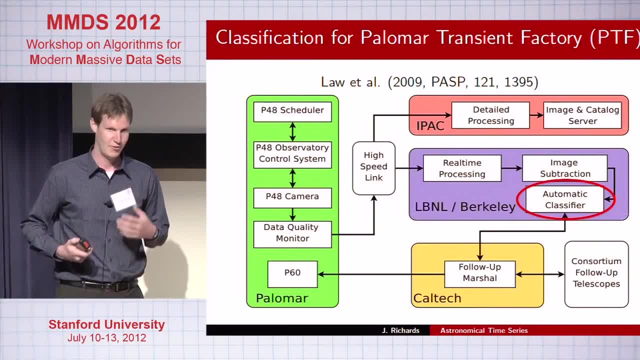 Variable stars will kind of pulsate and go up and down forever. So if it's a supernova, we want to, you know. we want to know if it's a supernova, is it a variable star? We want to send that information as fast as possible. 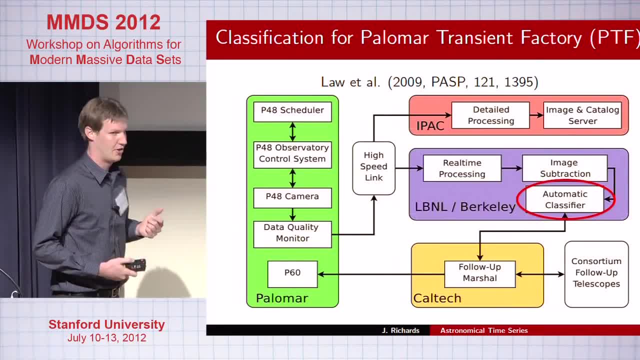 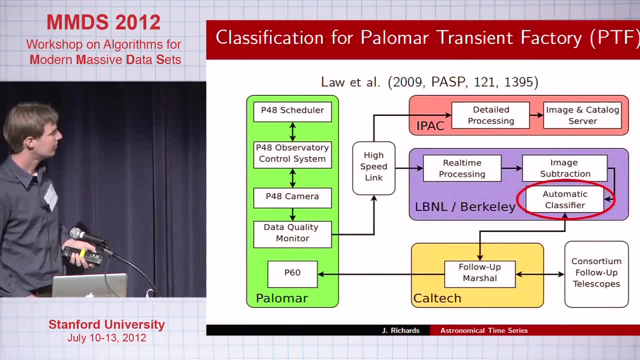 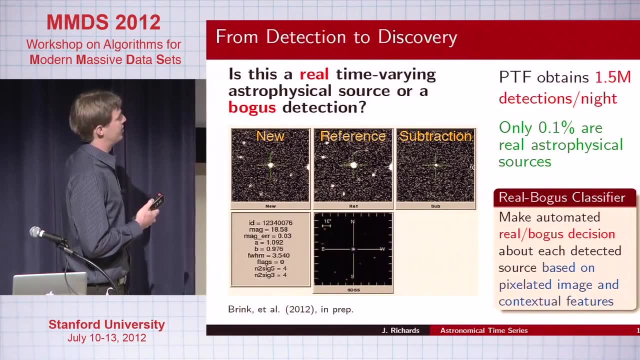 to Caltech, where they will decide whether or not to follow up with other telescopes to get more precise information on those objects. Right, so, as I said, the first classification task is this real bogus problem. So these are the type of data that are sent to us. 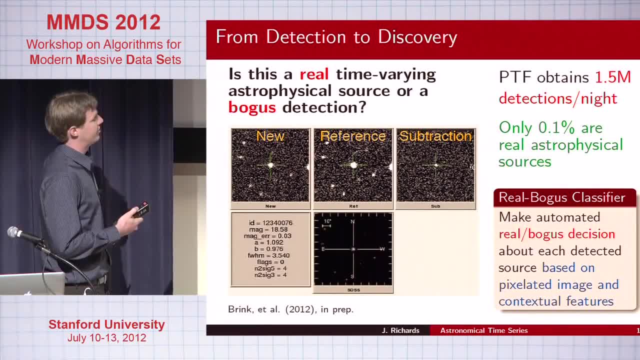 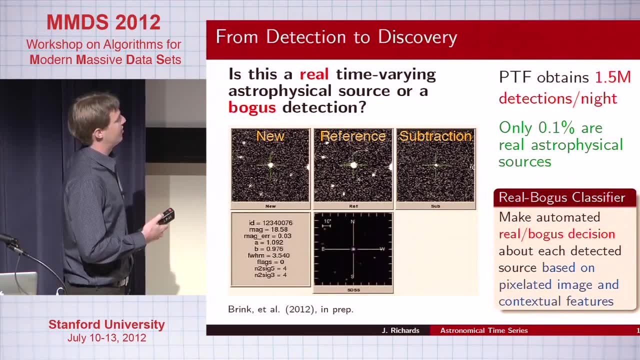 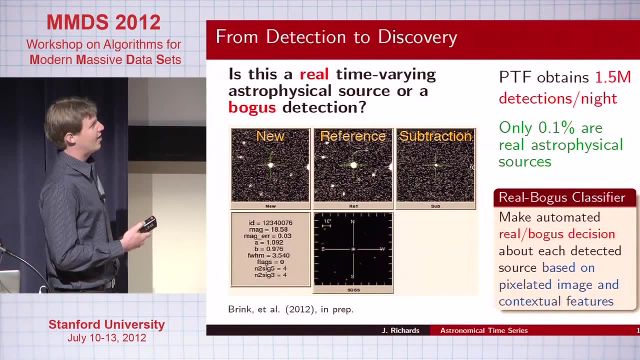 Here's the new image. This is a deep reference image. And then here's the subtraction. So this, this is real. Probably a variable star has gotten brighter over time, So it has a positive residual. It looks very clean. We're about 1.5 million detections a night. 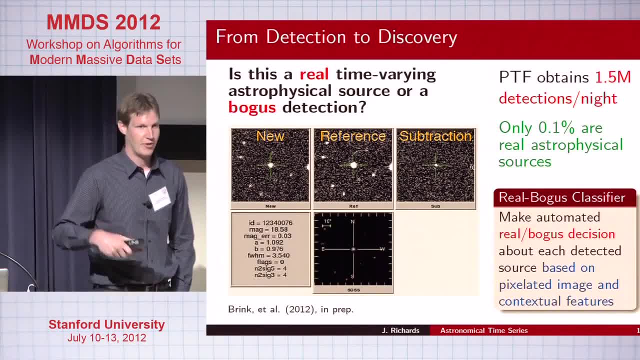 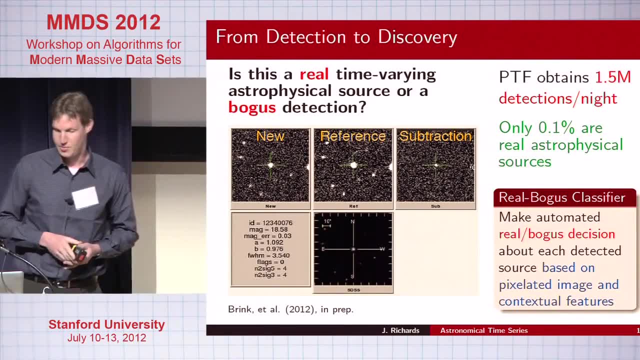 So anything that kind of pops up over some sigma threshold on the image is flagged as a detection. But only 0.1% of those are true astrophysically varying objects. So we made a what we call a real bogus classification. 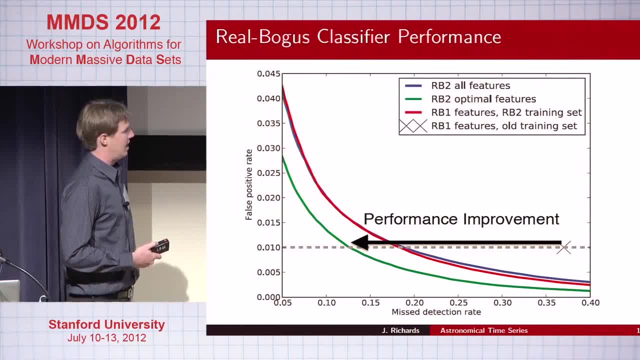 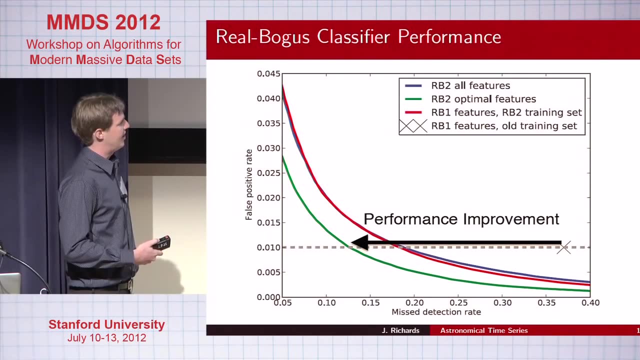 This is image plus some context features, And it uses a random forest classifier, which was the best out of about a dozen or so classifiers that we tried, And so we require a very small 1% false positive rate, And we see that from the beginning of the mission. 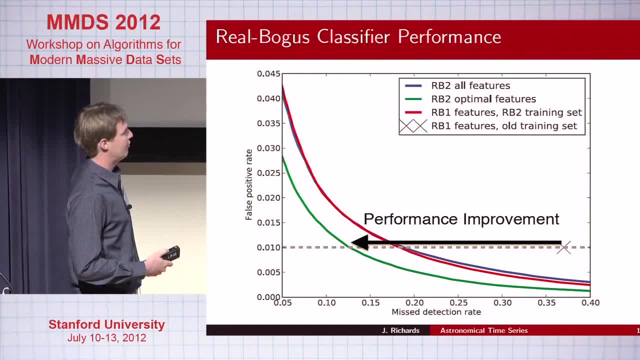 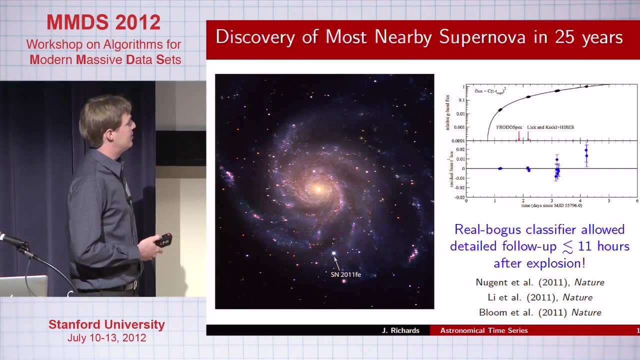 where our old algorithms were operating. we've decreased the misdetection rate of real astrophysically varying objects from the 35 to 40% down to about 10 to 15%. So mark a decrease. We recently- last year- found the most nearby supernova. 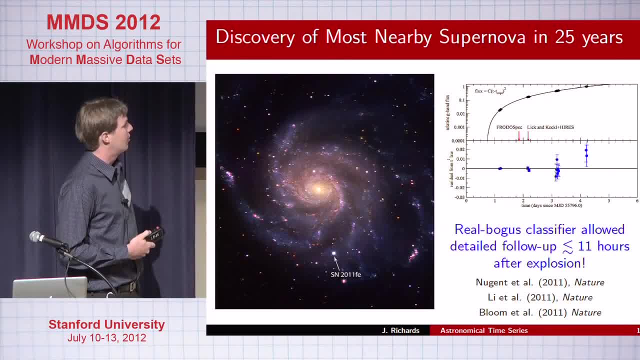 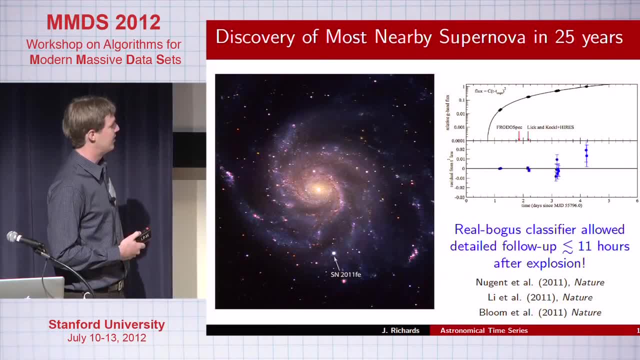 that's gone off in 25 years. So here's the pinwheel galaxy. It's about 21 million light years away from us. And here's the supernova. It's this big bright object And via this image subtraction and our classification pipeline, 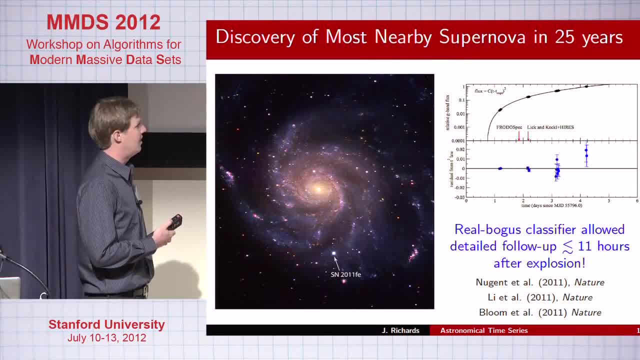 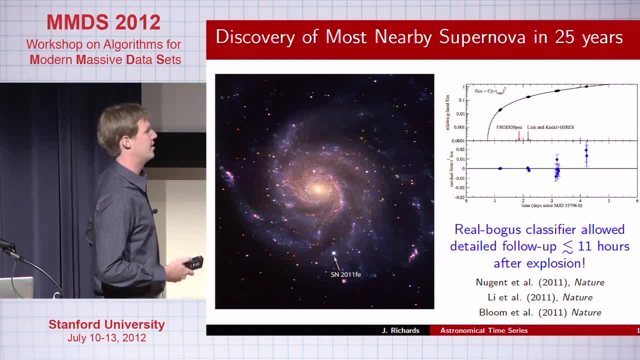 we were the first telescope to discover that the supernova had gone off. We weren't the first to detect it, but we were the first to actually turn that detection into a discovery, And this allowed us to do some detailed modeling of the explosion. 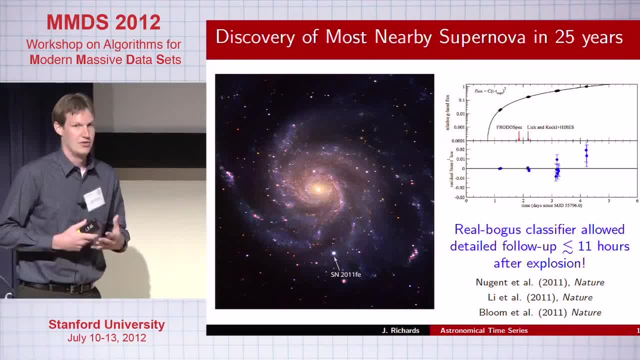 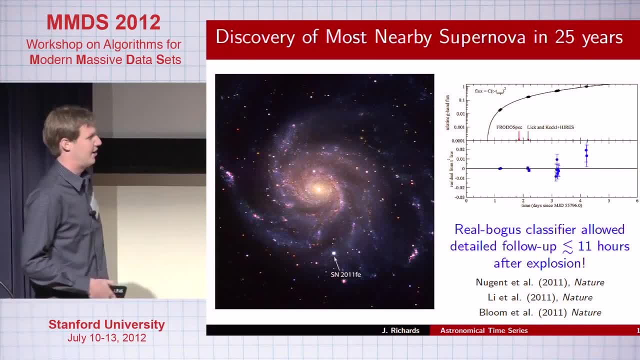 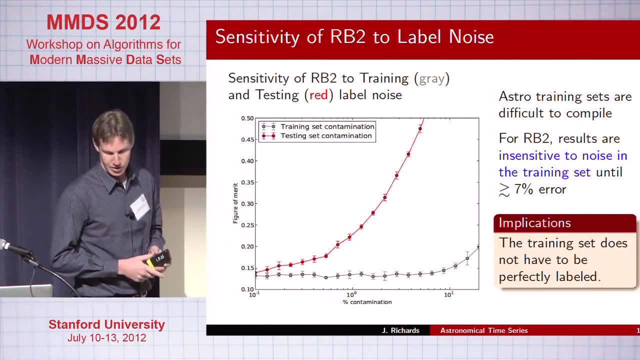 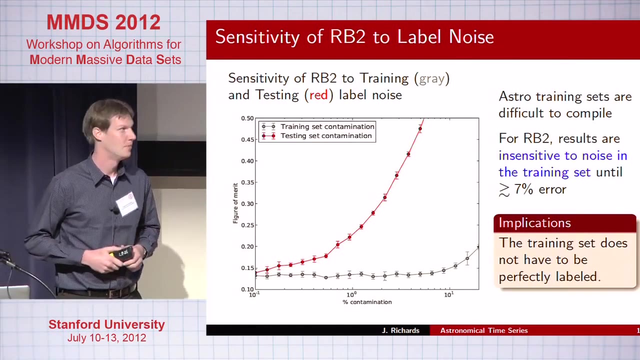 And we could basically constrain the time of the explosion to within an hour, which was unprecedented, And got to write several nature papers. As I mentioned before, one difficulty is in in doing these types of studies is getting clean training data. So spectroscopic followup resources are really expensive. 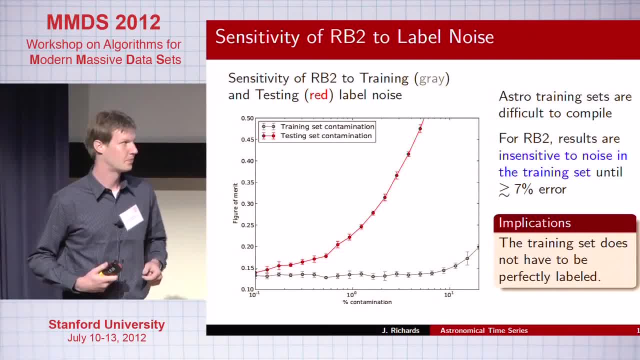 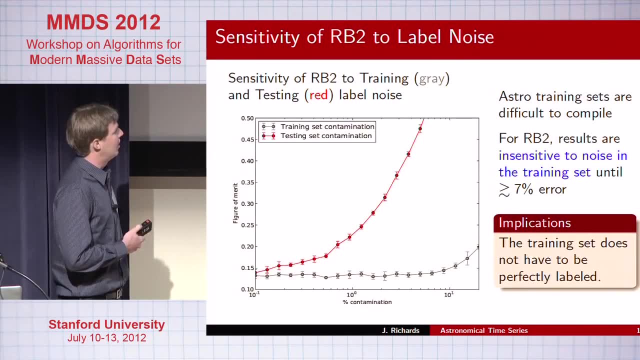 So you can't be going around following up everything that you think might be real. So getting an unbiased and clean training sample is extremely difficult. One result of this real, bogus classification is that we found, at least in our training set and with the random forest classifier, 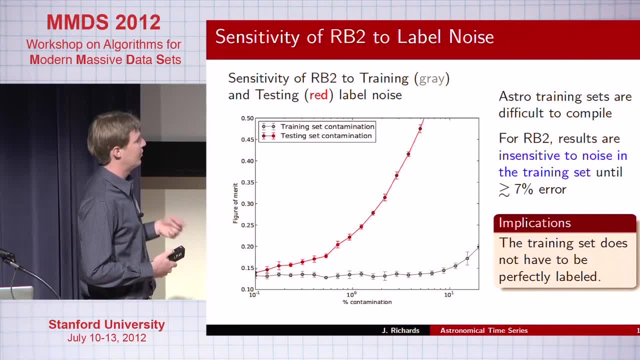 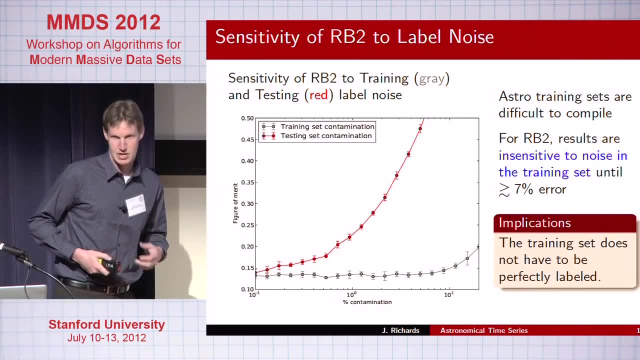 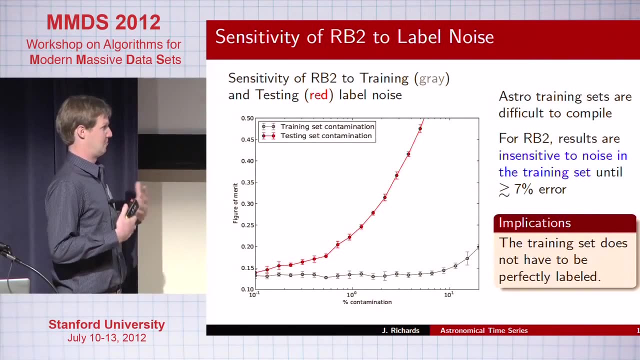 we're relatively insensitive to labeling errors in the training. set up to about a six or 7% level, We expect the contamination to be kind of sub 1%. So this implies that if we have a relatively good enough procedure and actually obtaining training sets, 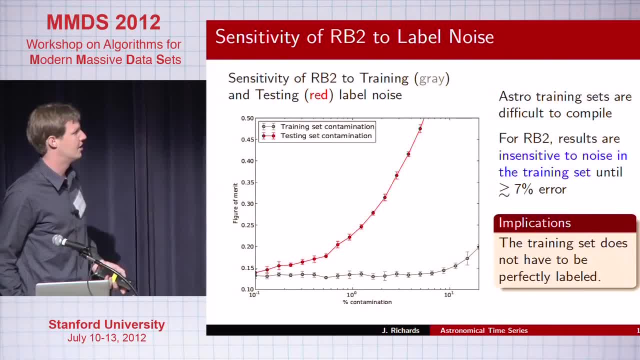 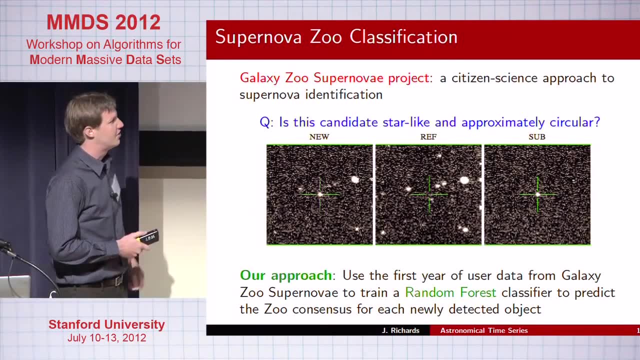 the classifier does a relatively good job at ignoring these errors. Another way to get training data is to use, you know, a little bit of data, And that's what we're trying to do. We're trying to use the public, So this is what's referred to as a citizen science project. 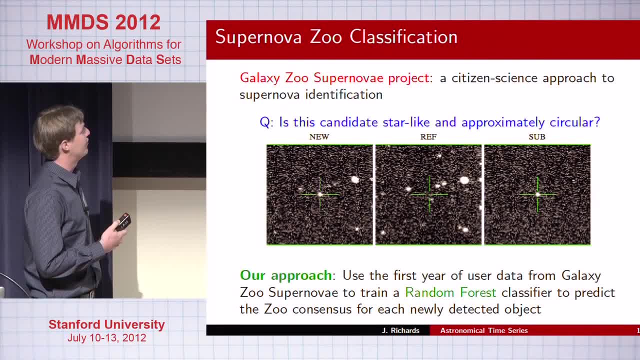 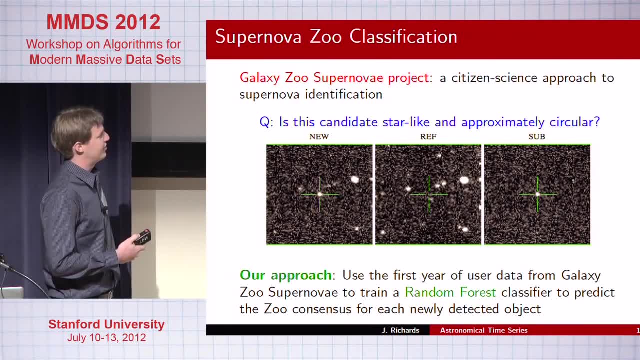 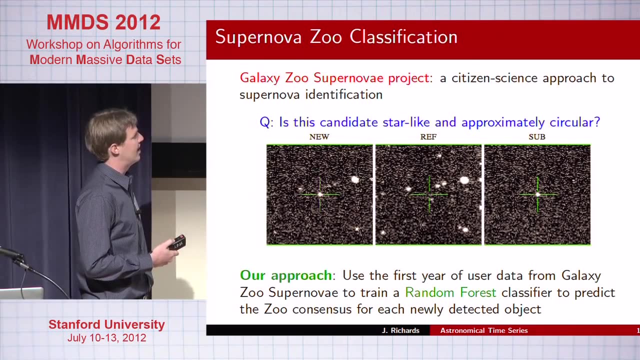 It's a part of the Zooniverse, It's called the Galaxy Zoo Supernova Project And basically the public can sign up and answer a bunch of questions about these supernova candidates, And so, over over about the course of two years now. 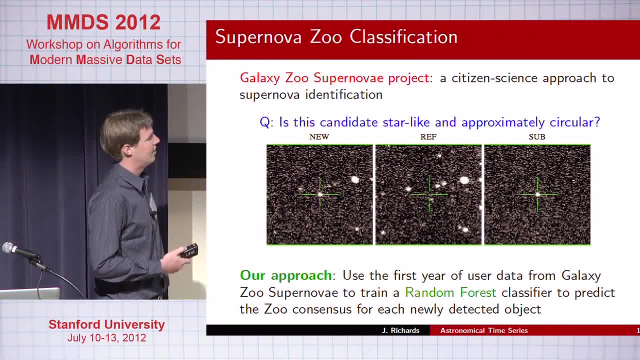 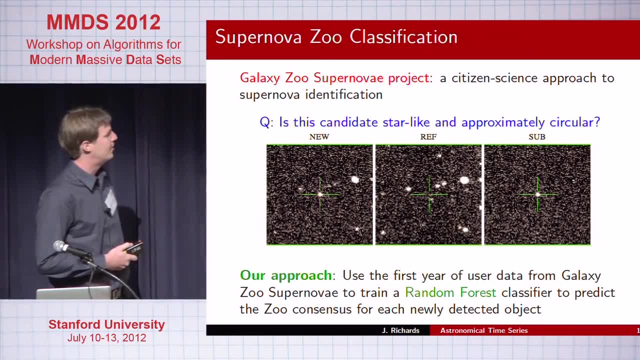 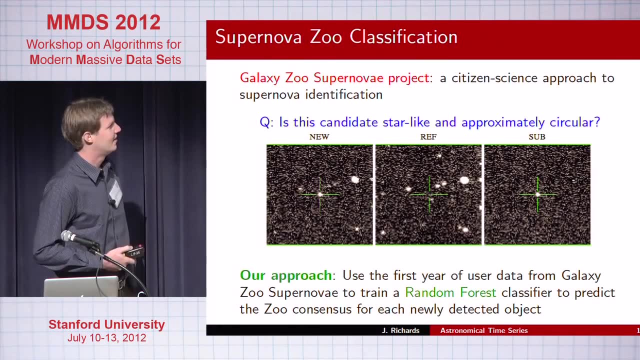 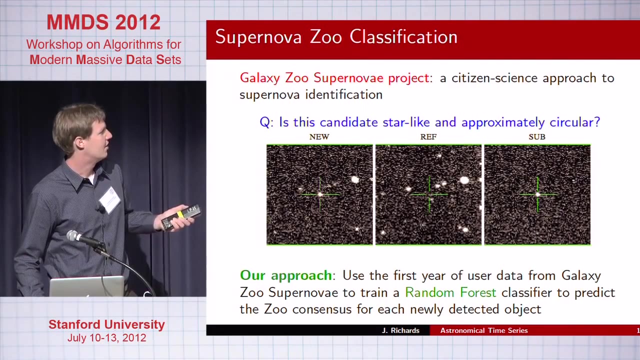 we have several tens of thousands of public monitored objects such as this. The public is pretty good, but they do miss certain objects. This is a confirmed type two supernova that, for some reason, the public did not think was real, And this is a very clearly real supernova. 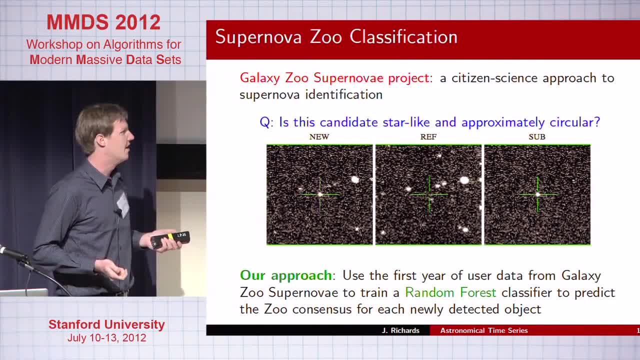 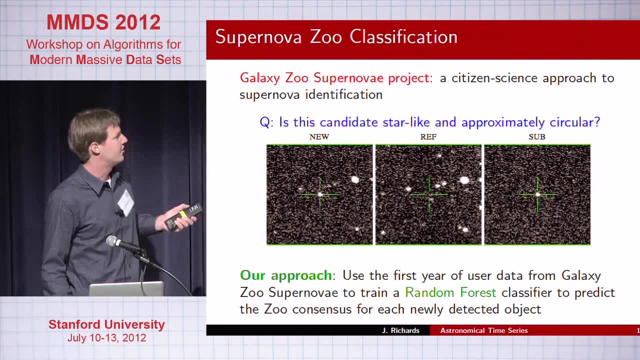 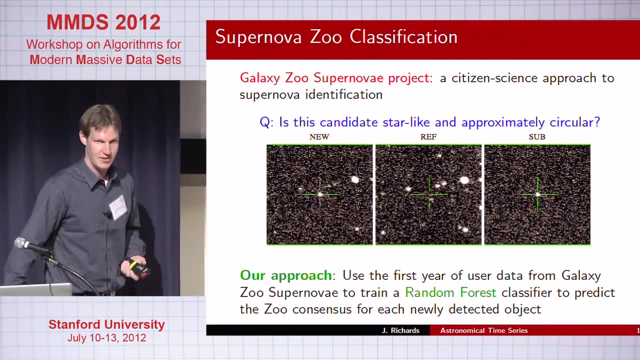 So our approach was to take this public data, these Galaxy Zoo supernova data, and actually build a random forest classifier to see features extracted from these images, plus some context information, to see if we could predict what the zoo would say hours before they would have time. 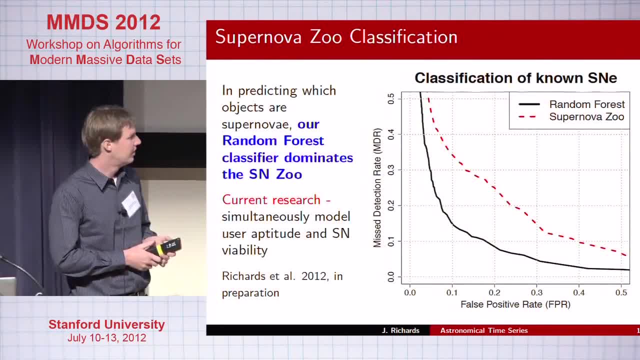 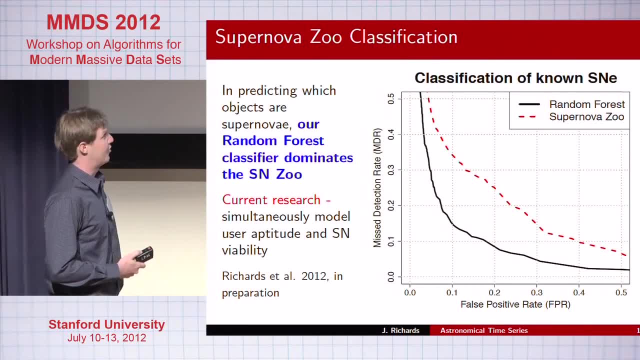 to actually look at each individual image And what we found is that we could do a pretty good job at predicting what the zoo would say, but, maybe more surprisingly, we did a better job at finding real supernovae. So these are the ROC curves. 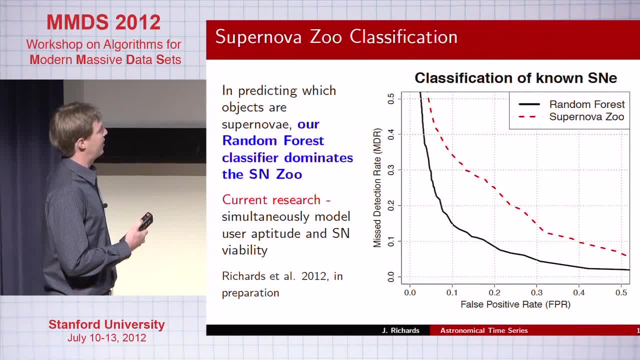 So the misdetection rate versus false positive rate- And the misdetection rate is the average of the classifier built just on the supernova zoo scores, versus our random forest classifier that was trained on the supernova zoo scores. And so it's kind of interesting that, even though we trained 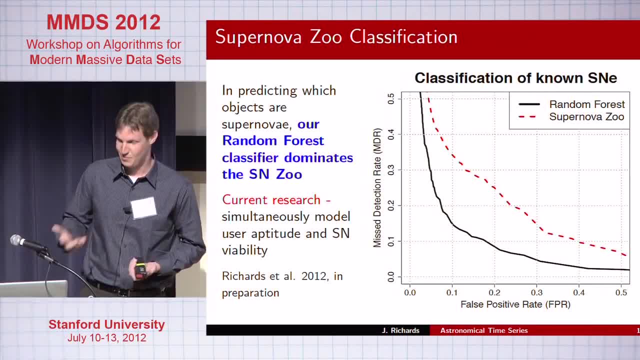 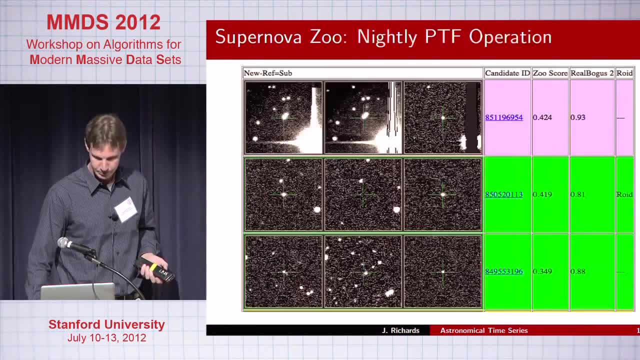 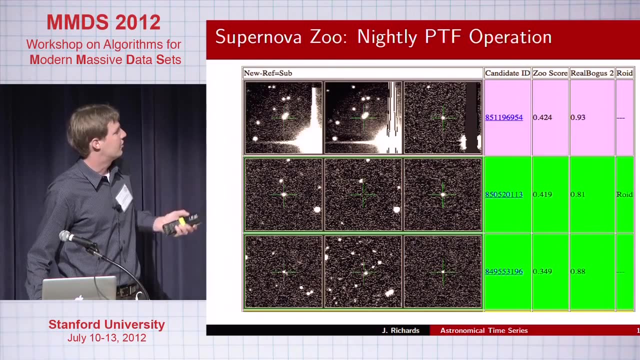 on their scores, because the machine learner does something kind of more in a self-consistent fashion, you actually get better performance overall on classification. And so now nightly we basically compute the zoo score and the real bogus two score for each of hundreds of. 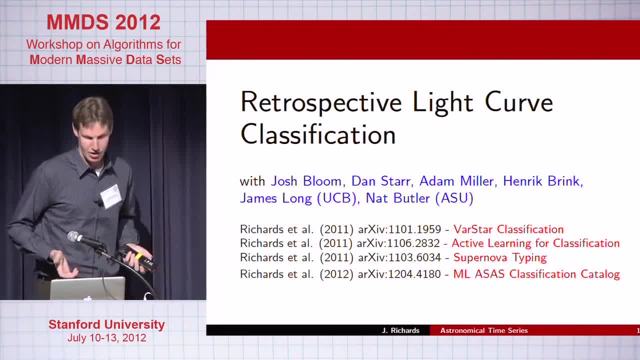 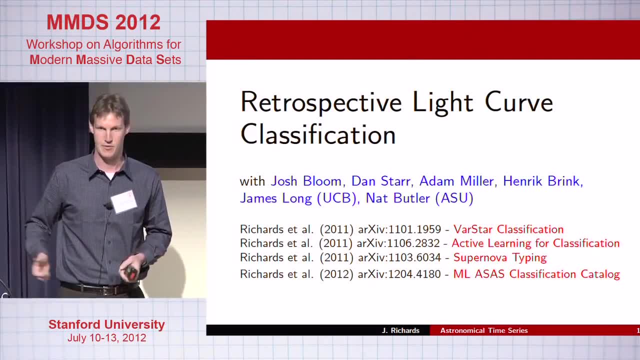 of candidates. Okay, so the second part is a little bit different. It's retrospective light curve classification. So, in other words, what happens at the end of the survey when we have all these times, this time series information? we've maybe followed up on some of the transients. 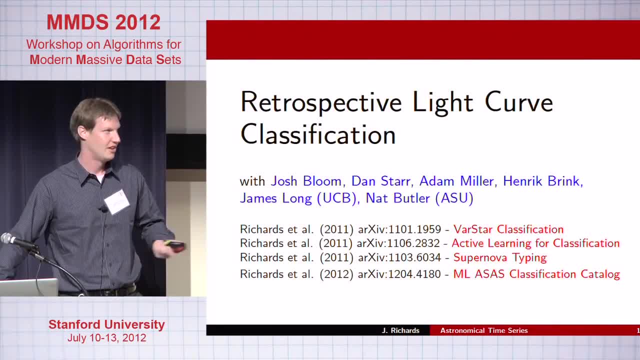 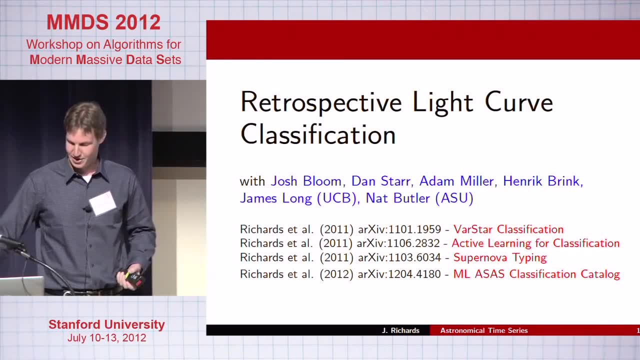 and supernovae that we could, and we have all these variable stars. The astrophysicists obviously want to do, want to use all the data in their data set. yet without good classification, it's a lot of, it's a lot of useless information for them. 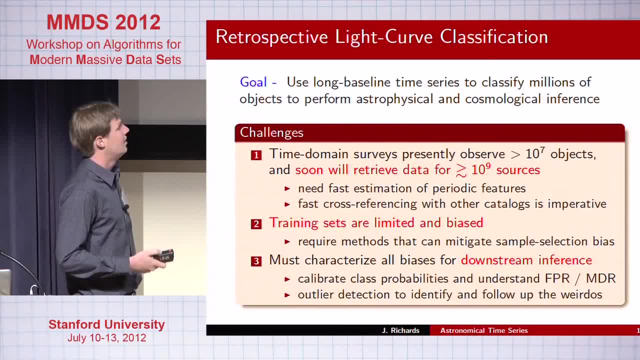 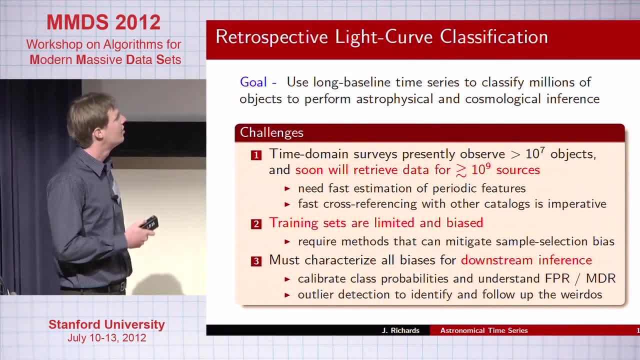 So the goal is to use these long baseline time series. So these surveys last typically from maybe a couple years up to 10 or more years. And so we have 10 years of data and say, and millions up to a billion objects- Right, so we need- we're talking about LSST- 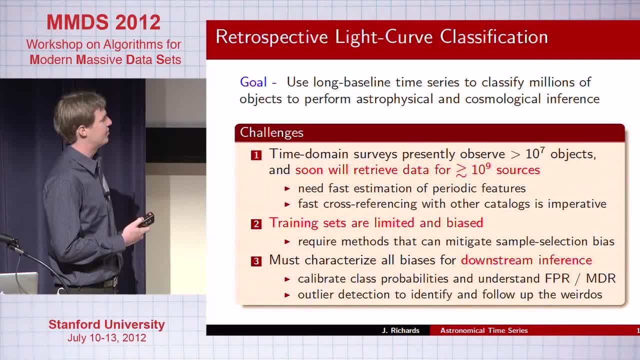 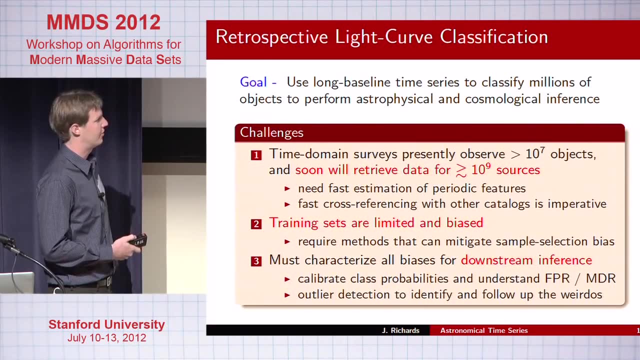 order of 10 to the nine sources. We need faster estimating estimation of features, especially periodic features. So for things that are periodic, the period is by far the best feature. Training sets, again, are limited and also biased, And I'll talk about that in a bit. This is a severe limitation for the work that we do. 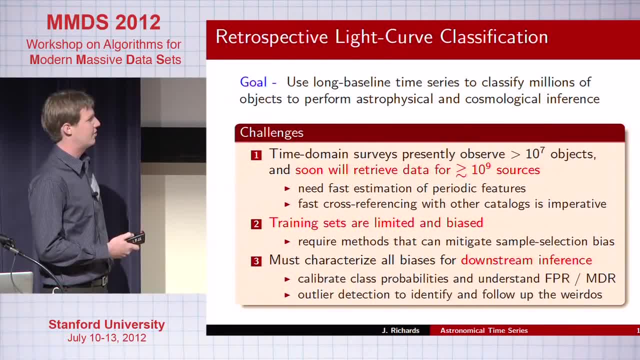 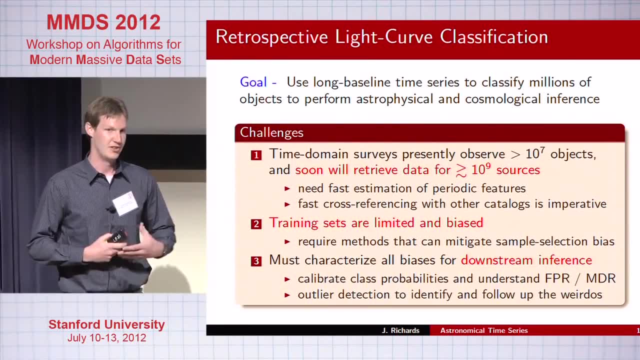 And these biases must be characterized for downstream inference. So typically if we're giving someone a classification of a survey, the astrophysicist wants to use it to infer properties of the universe. So what's the rate of type 1A supernovae within the local? 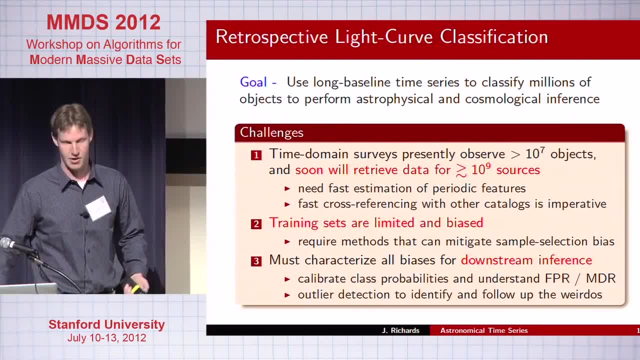 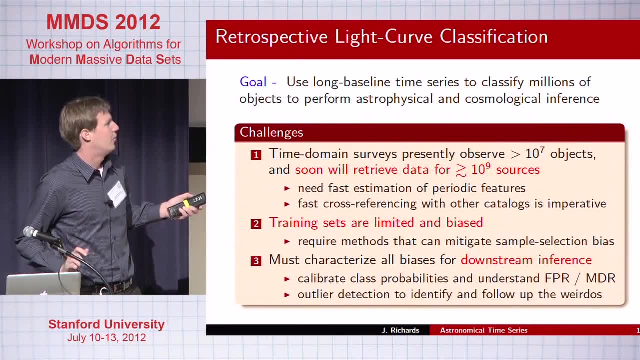 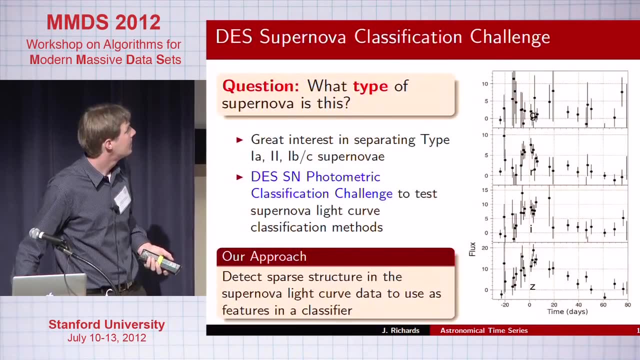 universe, What's the structure or what's the census of our library stores within the galaxy. So unless we understand all the biases in our training sets, plus our false positive and misdetection rates, these things aren't that useful for these timers. So one of the first. 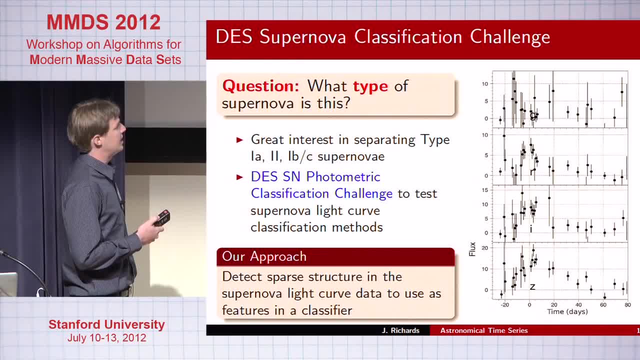 projects that I did with this type of data is taking. you know I'm not going to go into too much detail about this, but I'm going to go into a little bit more detail about this. So this is a supernovae. Now, instead of trying to determine is something a supernova or not at the 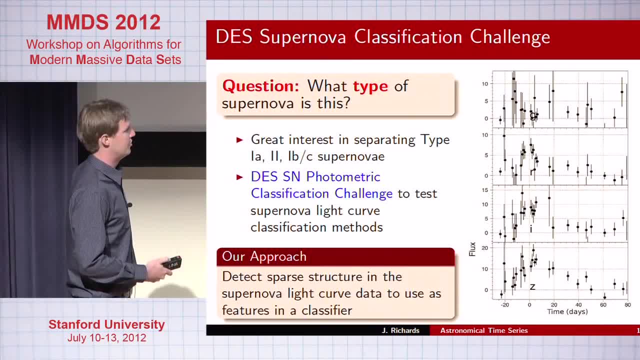 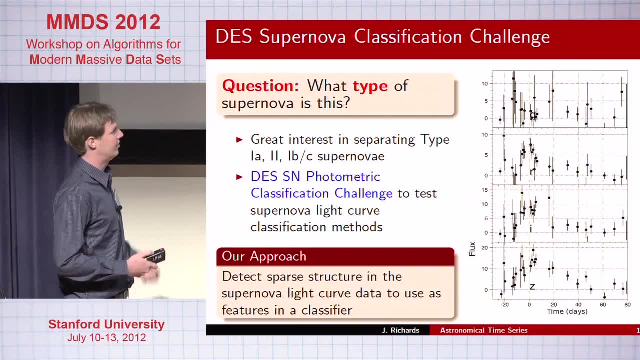 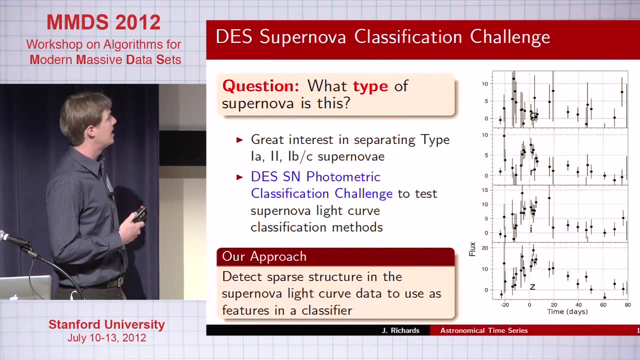 time of detection. now take, you know, a few months of data, once the supernova has exploded and faded away, to try to break them in the, to classify them into their subtypes. So there's, you know, about ten different subtypes of supernovae. People are typically interested in 1As but other 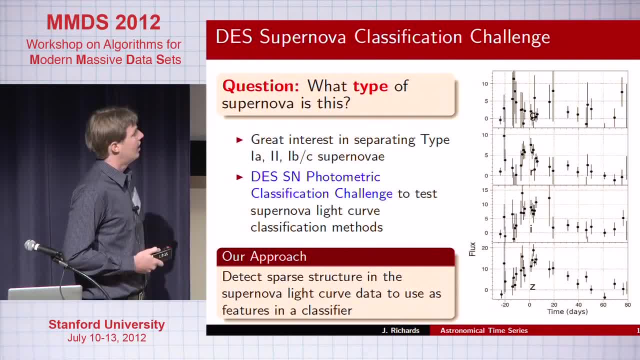 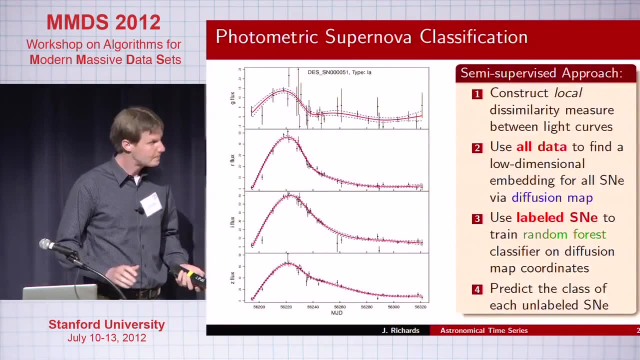 people are interested in different subtypes, And so our approach on this is- you know we're focusing on this- was to detect some sort of sparse structure in the entire database of supernova time series to do to build a classifier. So here again is: this is data for a single supernova. 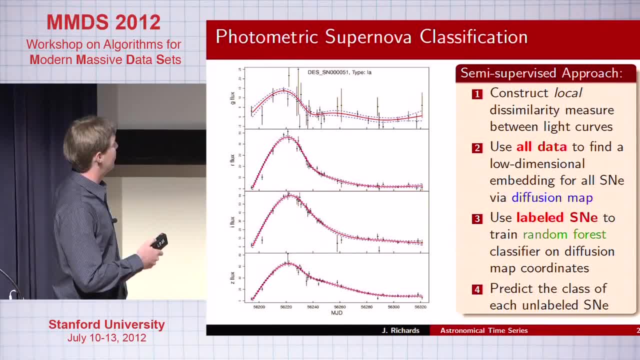 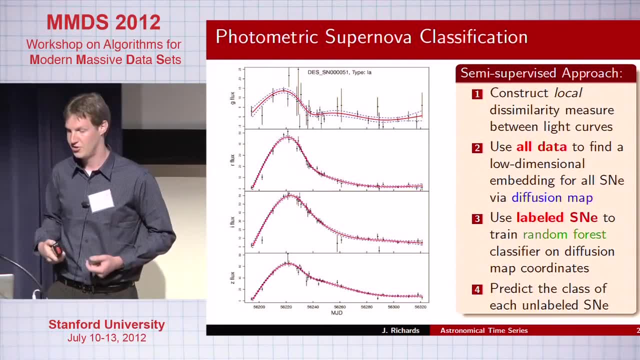 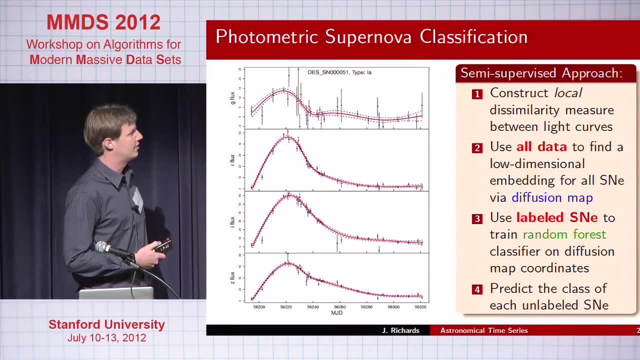 The data points are the black dots and then just a single spline model in each of the bands. So our approach was to construct some sort of local dissimilarity measure between light curves, then use the entire data set of the labeled plus the unlabeled data to find a low dimensional embedding. 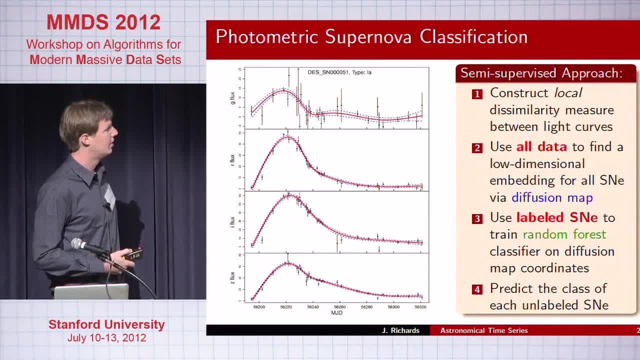 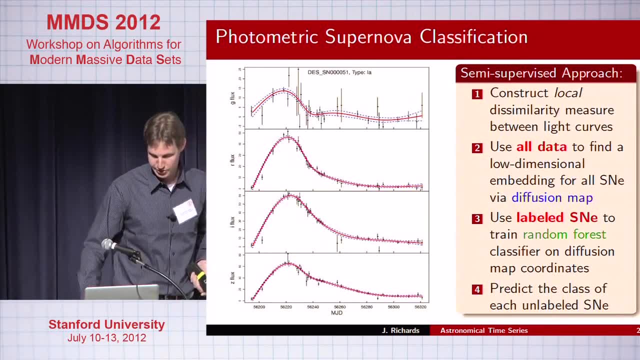 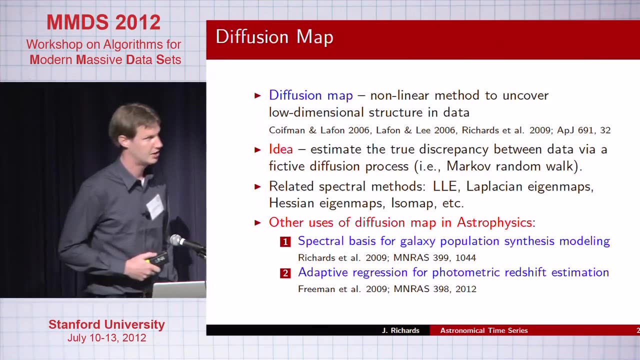 and we use a diffusion map, manifold learning method, Then use labeled supernovae to train a random forest and predict the class of each unlabeled supernova. So for those unfamiliar with the fusion map, it's a nonlinear dimensionality reduction technique. It's pretty related to 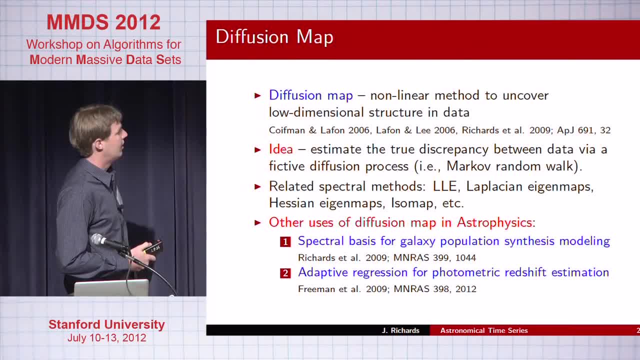 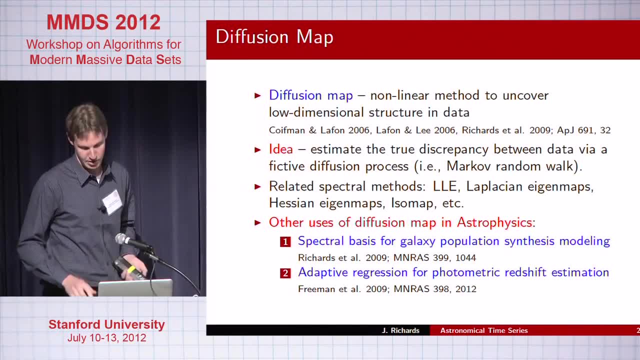 Laplacian eigenmaps- local linear embedding Lafon and Koifman, and Lafon and Lee wrote papers in 2006 on the method And we've used it in a variety of astronomical applications. The general idea is assume we have some data in two. 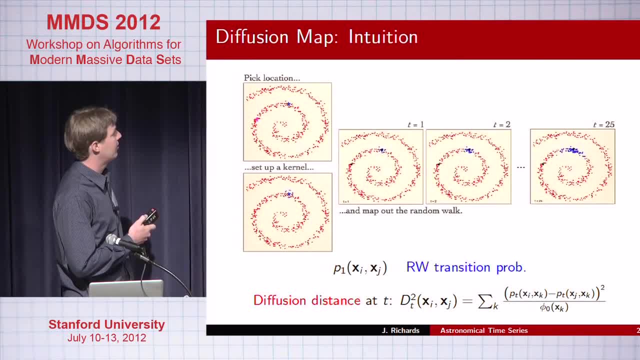 dimensions, set up a local kernel around each data point and now run a fictive diffusion process where you're only allowed to jump to nearby data points. And if you map out this random walk, the distance between your conditional probability vectors is a really robust description of the true 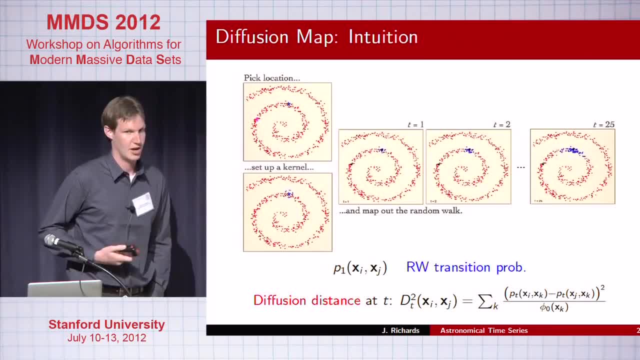 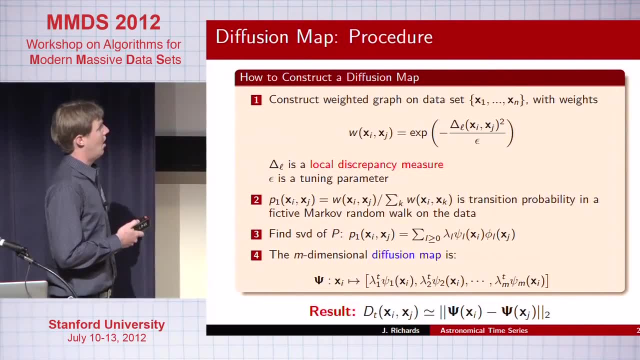 distance in your data set with respect to the geometry of the data, So in higher dimensions. this is a pretty useful technique. It's relatively simple: Just set up a weighted graph on your data, So each data point here is a time series for a single supernova. The weights are: 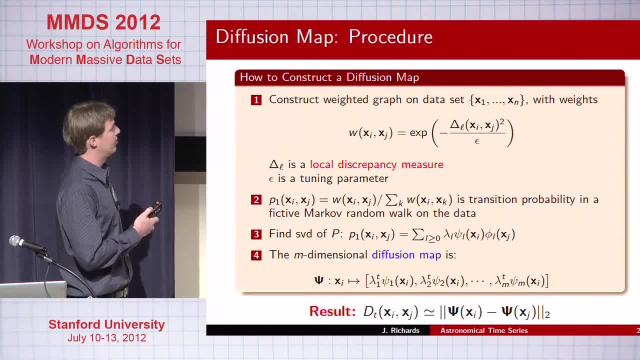 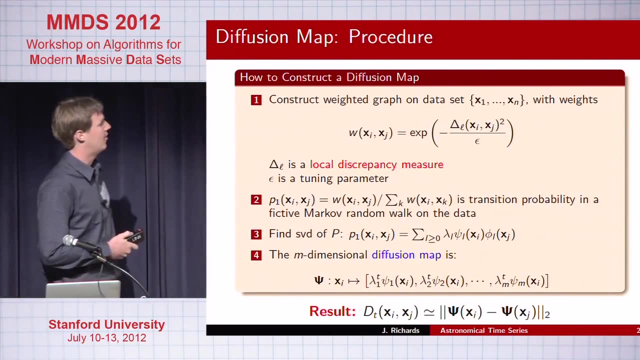 different. We just use a Gaussian kernel with the local distance discrepancy measure you can pick, And epsilon is a tuning parameter. Now normalize these to row, sum to one And that's a transition probability matrix of a Markov random walk. And if we take the bi-orthogonal SVD of this P matrix, 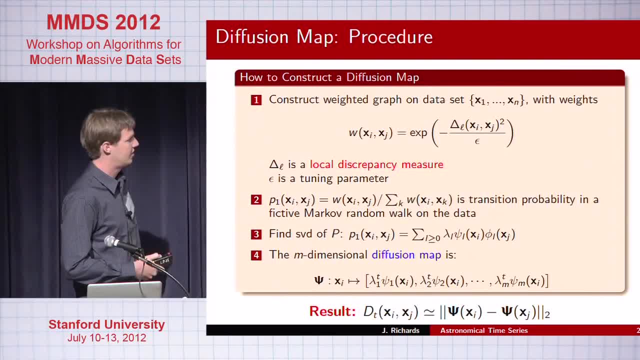 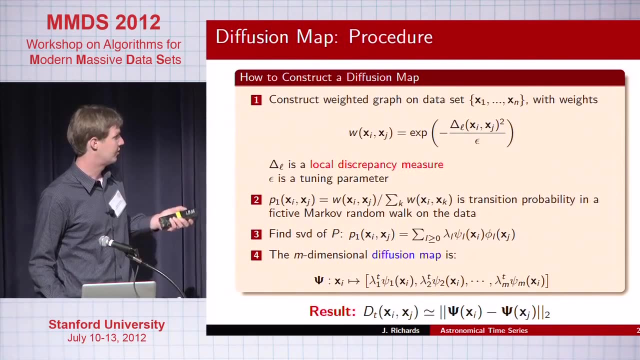 then the projection of the data onto the space defined by these eigenvalues and eigenvectors has a property: that Euclidean distances in that space are approximately equal to the diffusion distance, which really capture dissimilarity in our data. So we use these coordinates as features and a 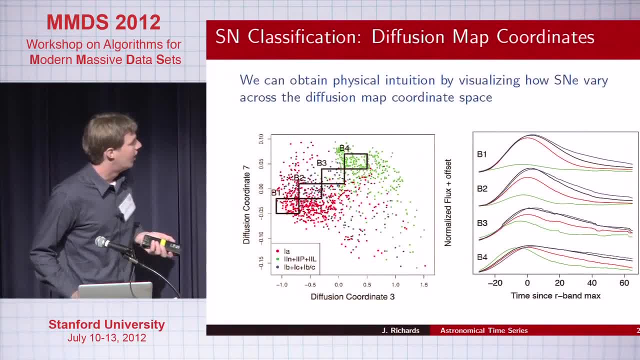 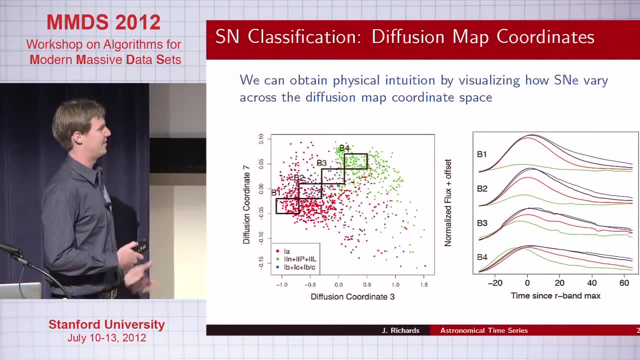 classifier Even prior to doing classification. the astrophysicists are always interested in physical interpretation. They want to know what diffusion coordinate seven means, and I tell them: you know, you don't really. it has no meaning. You just have to look at what the light curves look like, as you. 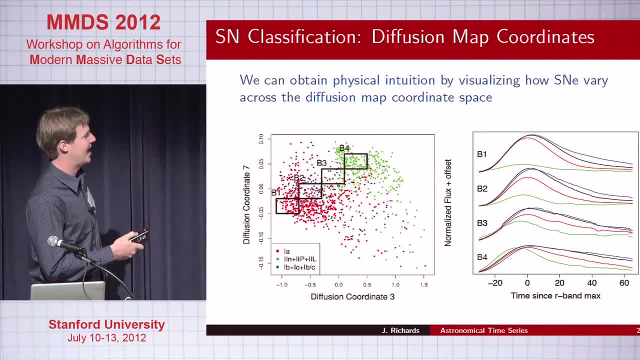 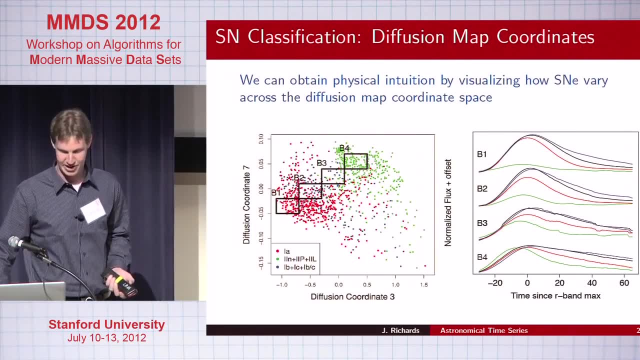 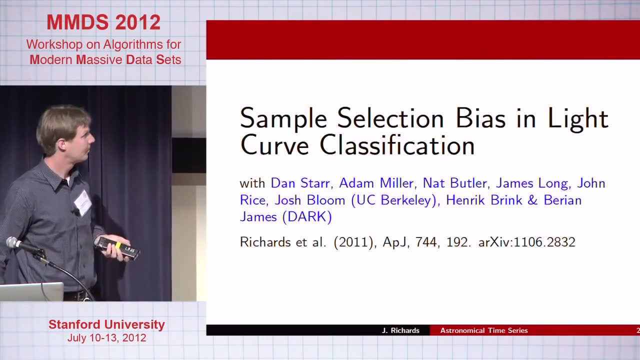 step across this space. So we can do that, and they're pretty satisfied with how these average light curves look. But if the ultimate goal is prediction, then we can build a classifier in this high dimensional space and we'd actually do pretty well. Interestingly so, this data set is quite interesting. 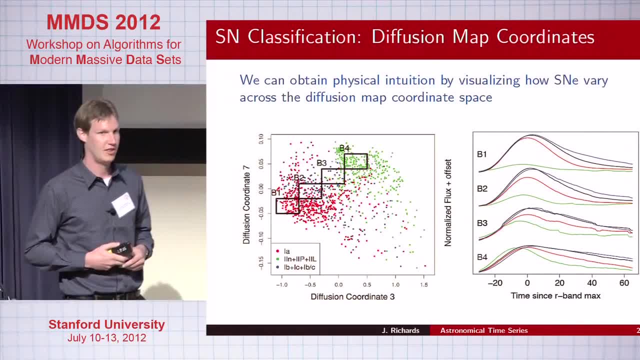 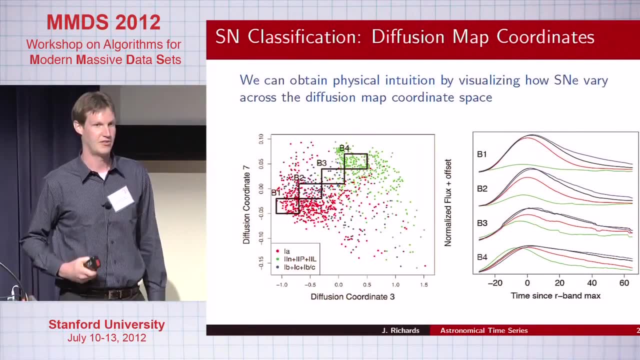 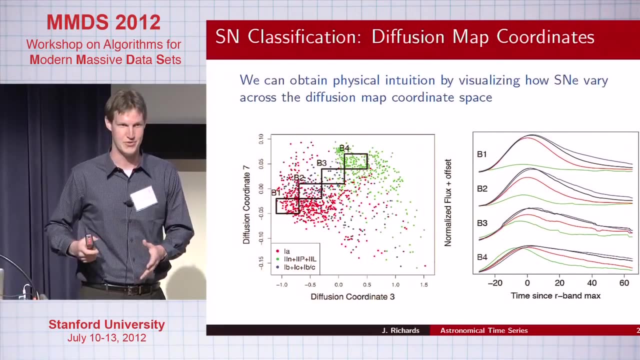 It was one of these data challenges that was run by the dark energy survey and they wanted to basically compete all these different classifiers against one another, And so about half the people use kind of standard non-parametric tools. The other half use physical template fittings. They have these physical 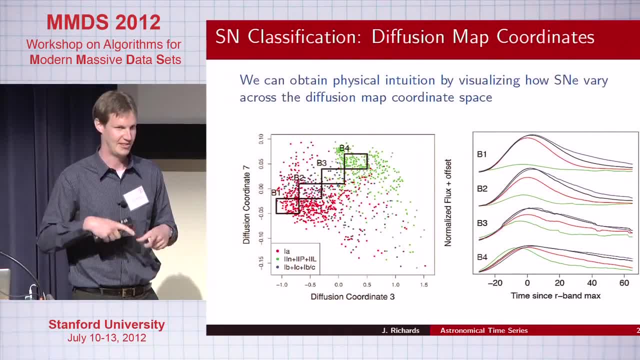 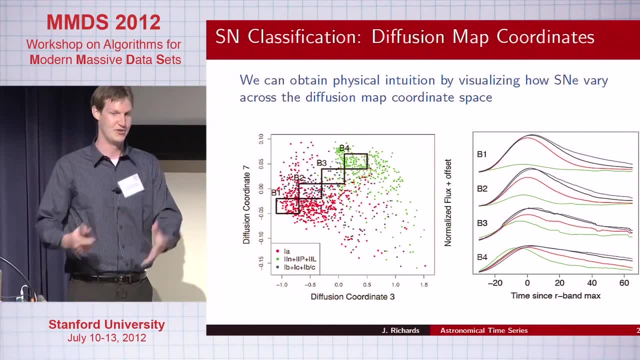 ideas about what time series what these light curves look like And even though the data were generated by kind of similar template dictionaries, they didn't really know what these light curves looked like. They didn't know what time series were used by many of the teams in doing the fitting. There wasn't a drastic 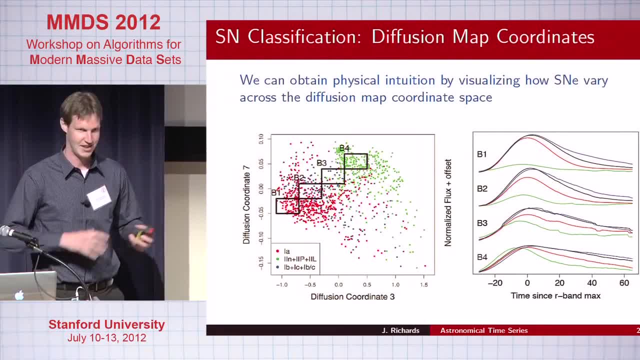 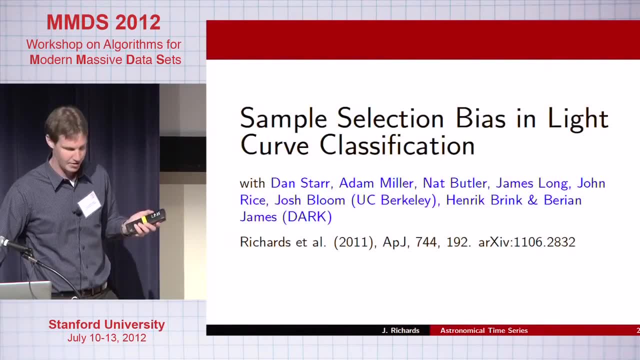 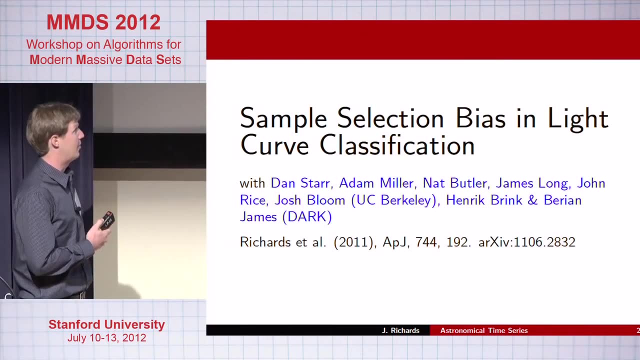 difference between the non-parametric methods and the actual physical fitting methods. So that was pretty interesting. But anyway, one of the, if not the most challenging aspect of this sort of classification is sample selection bias. So the training sets in astronomical applications are extremely biased and I'll show. 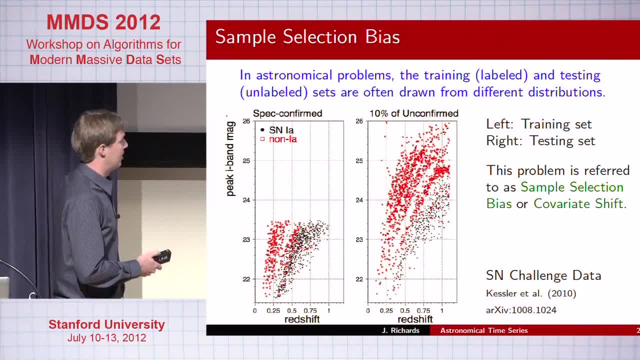 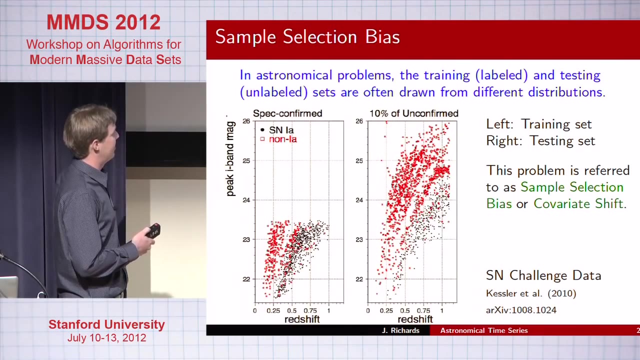 you an example. Here are the data again from the supernova challenge. On the left: here I plotted the kind of peak magnitude, so the brightness, the peak brightness versus the redshift, so the distance, And here astronomers are weird. so lower numbers means brighter. So our training set consists of these extremely bright 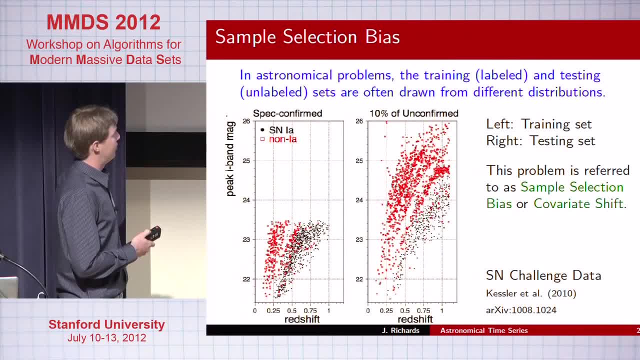 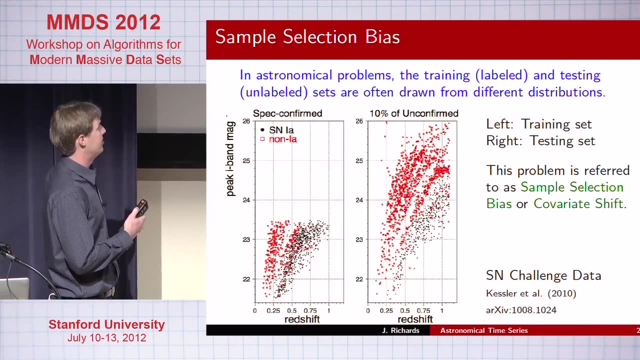 relatively local supernovae, And so the task is to build some, you know, non-parametric or semi-parametric model on these data, to then classify this set of unconfirmed sources, And the limitation here again is spectroscopic observation. So spectra 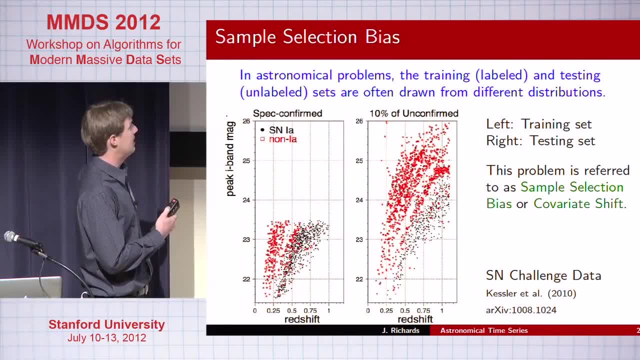 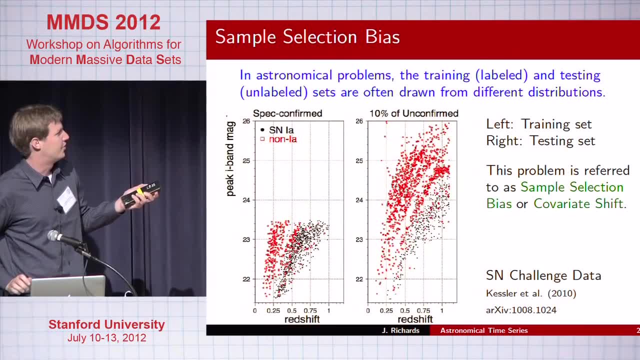 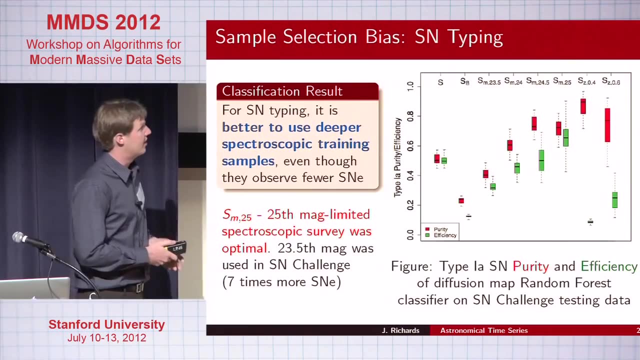 are extremely costly to get, especially as you go to fainter and fainter sources, And so this problem is referred to either sample selection bias or covariate shift, depending on what field you're in. And we show with this data set that if you assume a fixed amount of spectroscopic follow-up time and 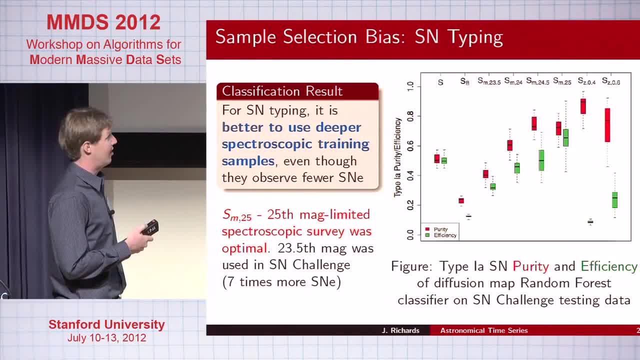 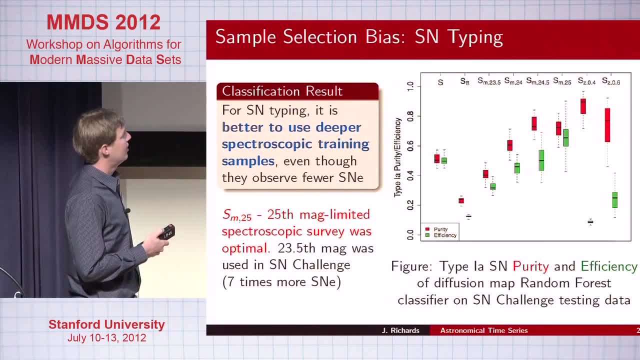 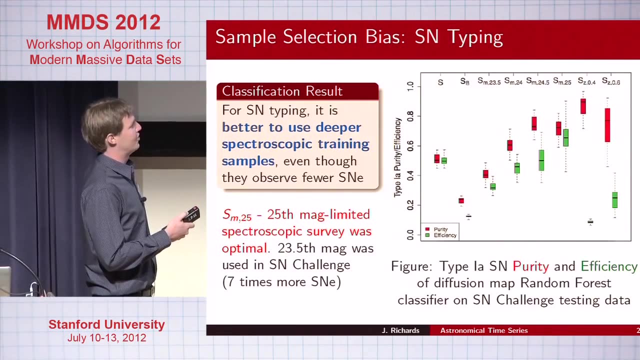 basically run different spectroscopic surveys with different magnitude limits. so here, as we go to the right, we get fainter and fainter. we actually get better performance in terms of purity and efficiency with the fainter limits, even though you're observing much fewer objects. So your training set size is. 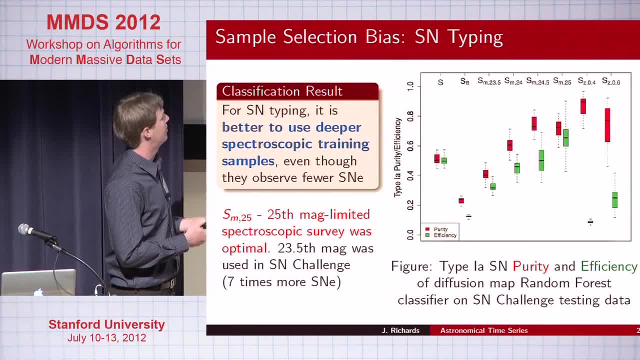 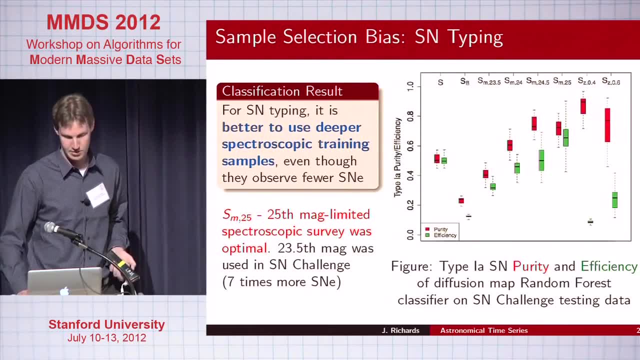 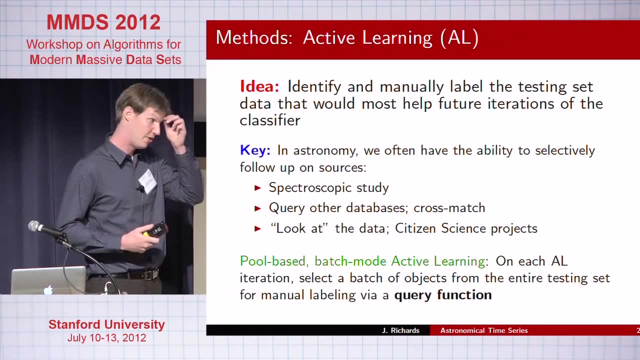 much, much smaller, maybe, I think, a seventh of the size as this one, but your performance in terms of purity and efficiency is much higher. I'll just skip ahead. So this causes us to look at other methods for trying to alleviate these types of biases. We found that active learning is extremely appropriate. 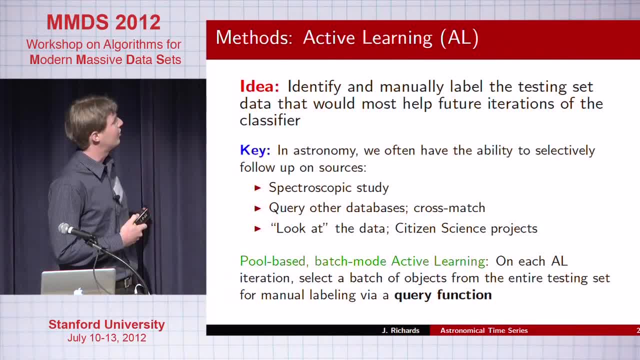 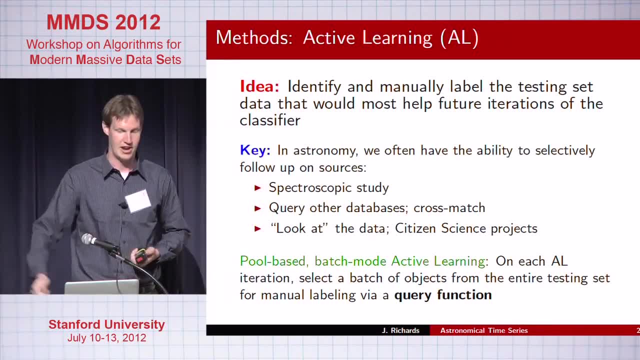 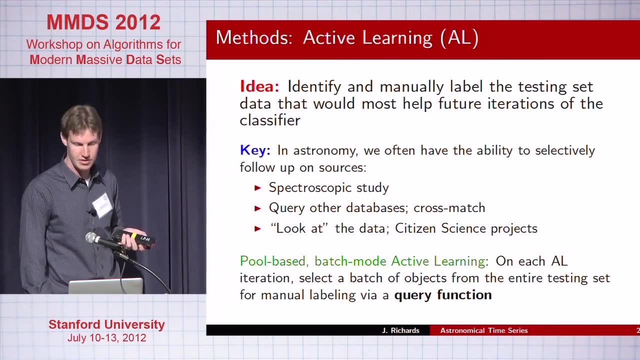 And so in active learning, if you're not familiar with it, the idea is that the classifier identifies the set of objects that would most help the classifier in further iterations, And the key is that we can judiciously follow up sources. So we want to follow up the sources that have the highest leverage in our 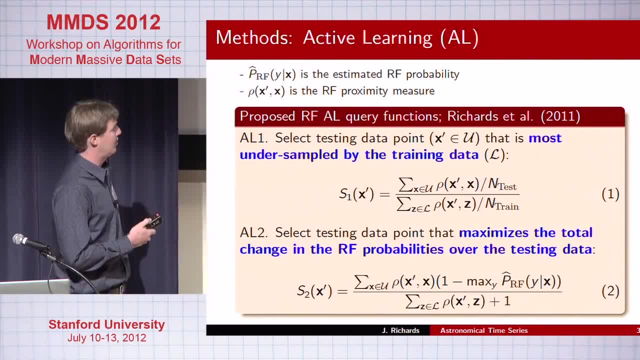 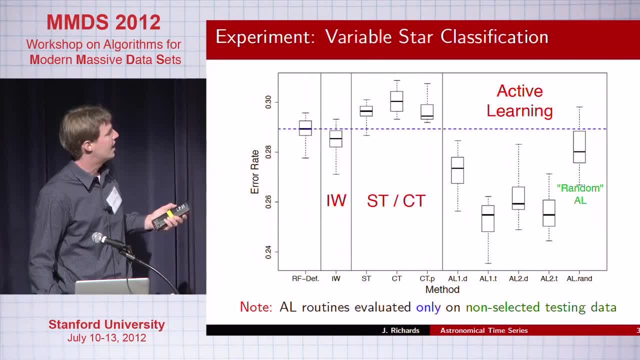 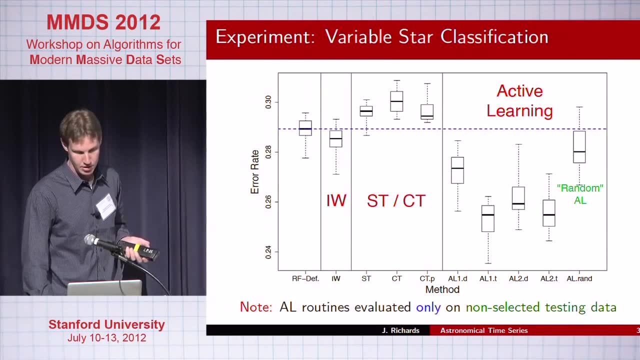 classification Using a random forest. we came up with a couple of heuristics for active learning And on some simulated data sets we showed that, compared to importance, weighting, self-training and co-training, it was the only method that produced any substantial gains in classification rate. 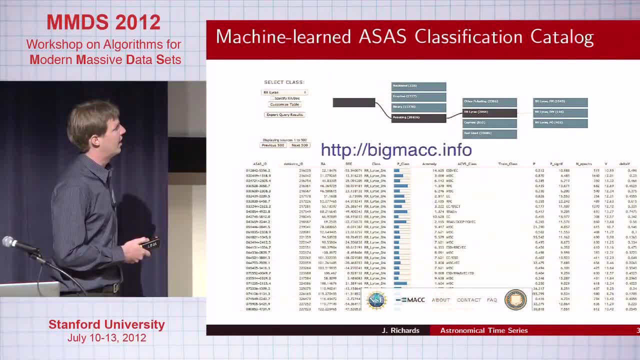 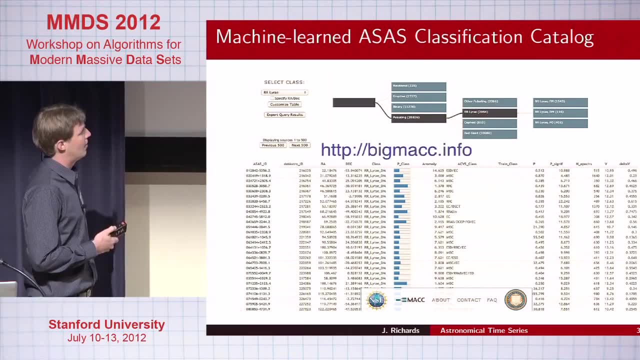 Let's skip ahead, And we recently put out a catalog of this survey called the AllSky Automated Survey. So it's a classification into about 30 different types of variable star And it's kind of the first catalog of its kind to actually give a probabilistic classification of astronauts. 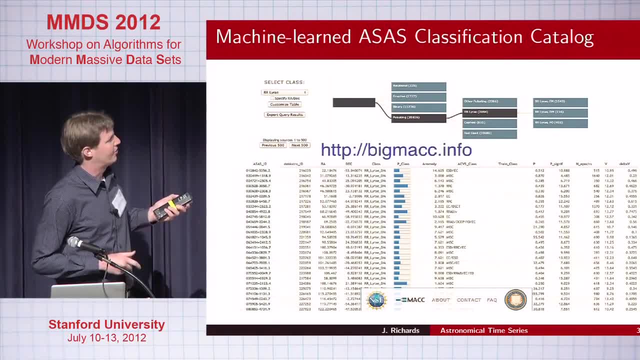 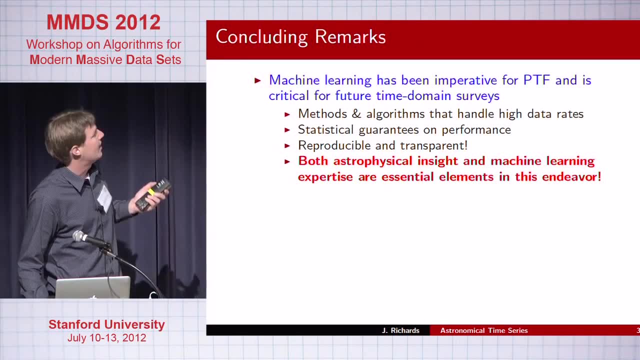 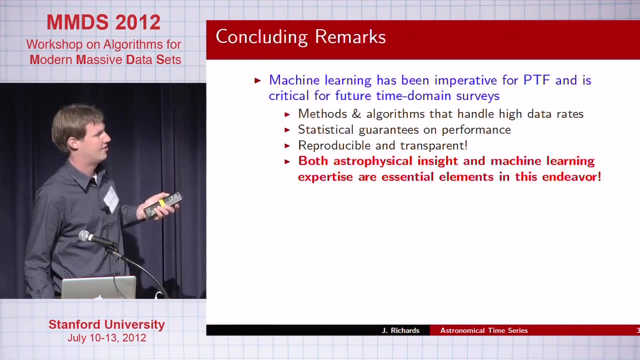 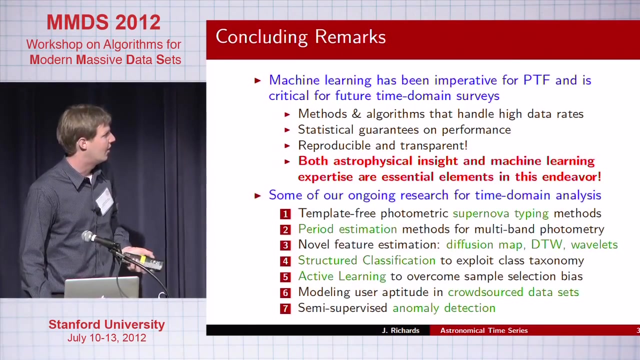 And it's very useful. So I'll just end by saying that machine learning has been critical for all this, but both astrophysical insight and machine learning are essential And I think having collaborations between different fields is really imperative. And I'll end there and take any questions that you have. 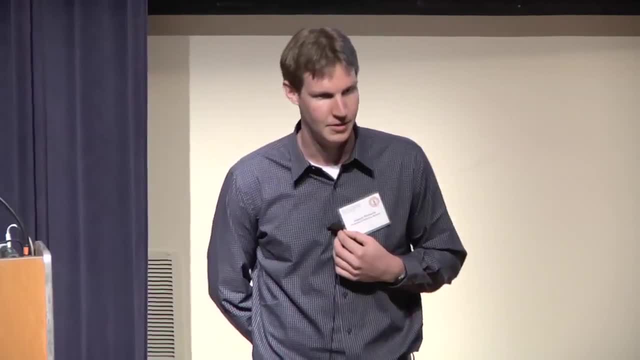 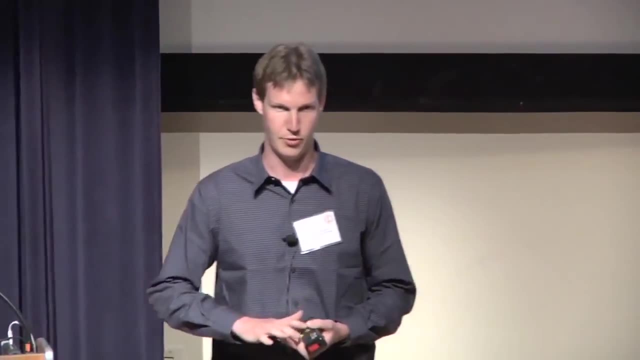 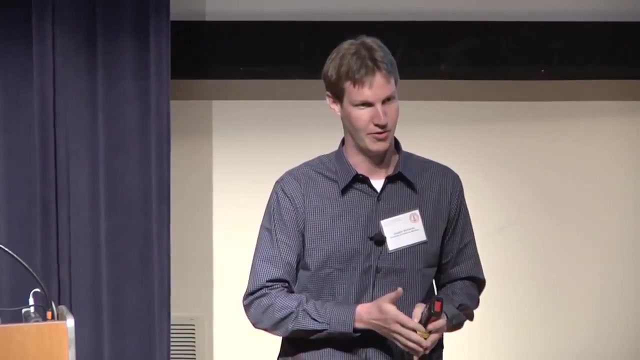 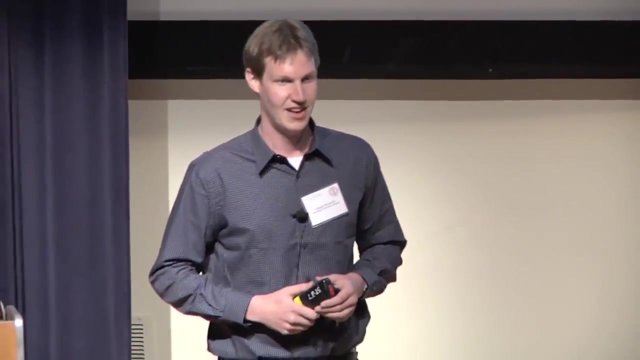 Okay, So I think the question is. so, prior to doing any of the classification for the Palomar Transient Factor, we do an image subtraction And I think she was wondering if there are any artifacts in the image or varying conditions of observation that need to be taken into account when we do this. Is that right, Yeah, So yes, We don't do that. 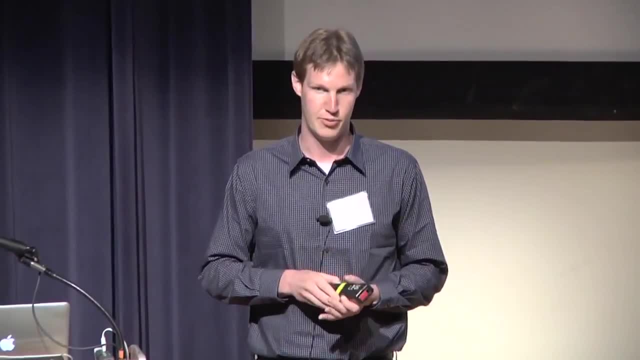 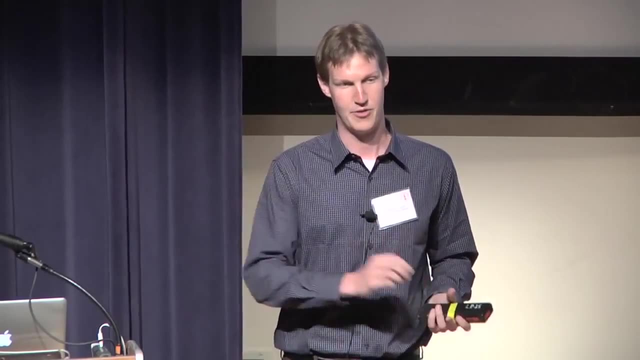 This is done by people at Lawrence Berkeley Lab But they have some pretty sophisticated data, But they have some pretty sophisticated tools for. so what happens is that the point spread function, so basically the smearing function, can vary from image to image. So they have to basically try to estimate that.